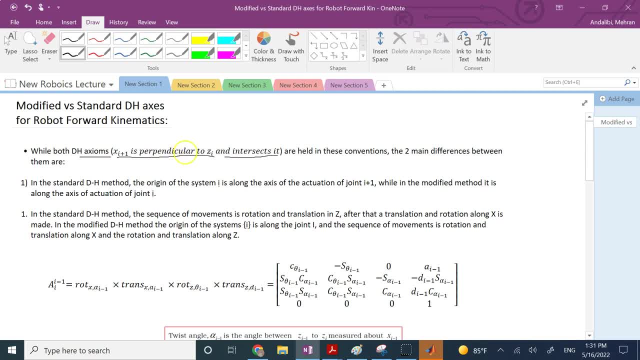 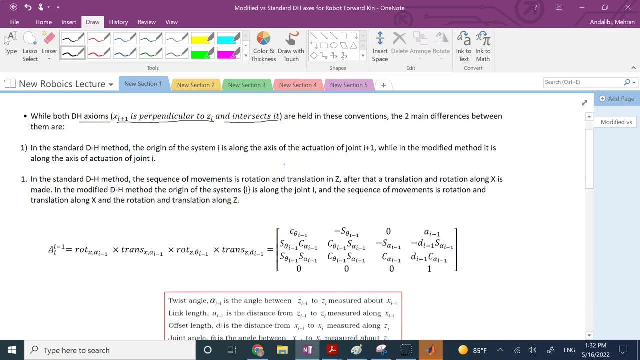 three for translation and three for rotation. But since you have two constraints or two axioms, two conditions, then all you need, instead of six parameters is to use four parameters. right, And if you go back and look at the video I made on my channel, you see, these four parameters are what we call. 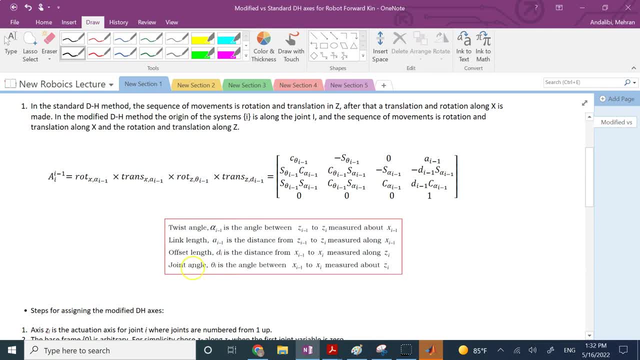 A, alpha D and theta right. We call them the joint parameters: angle, the joint or the land, the joint offset, basically, or the length of offset length, the length of the link, and the angle, the twist angle, alpha right. so we only need four parameters and 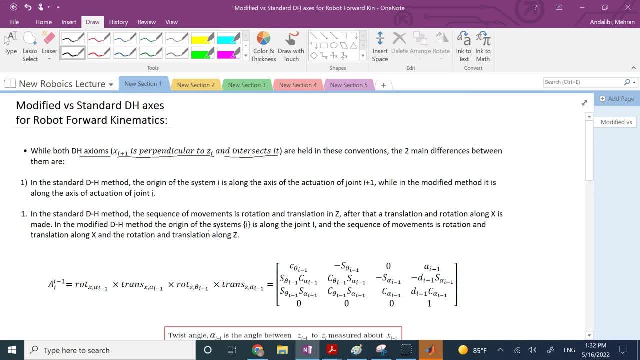 that's the one of the good things, the important things about the edge is it tries to use a minimal set of parameters to describe going from one frame to the next- four instead of six- by applying these two axioms. so we're still going to have these axioms in the modified frame, in the modified 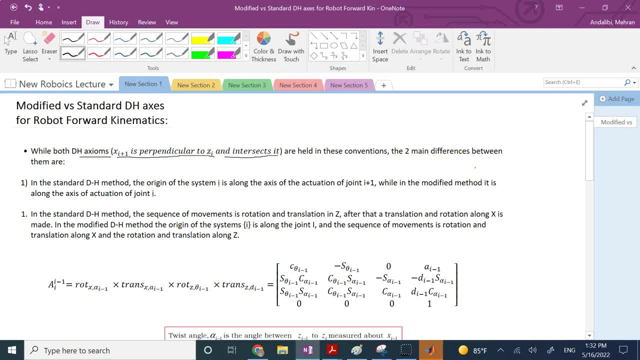 convention. but the modified convention is different from the standard in what, in two major ways, one- this one- is actually the advantage, i would say, of the modified convention over the standard. this first difference is in the standard. if you remember, the axis of actuation of joint i plus one was called z i, so frame i and z i. basically z i is the actuation. 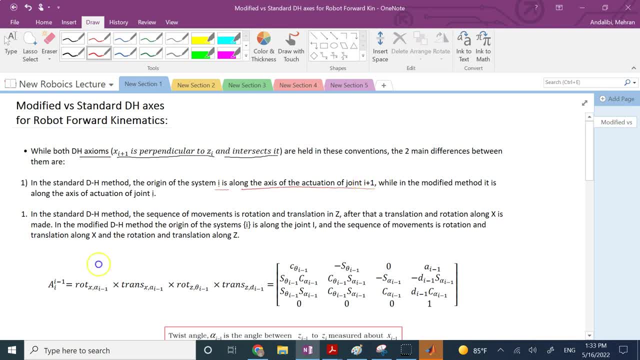 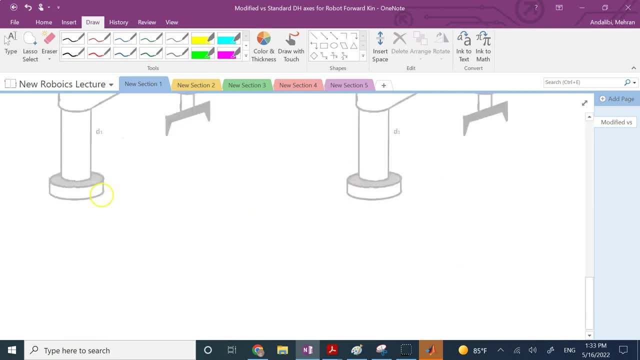 axis for joint i plus one. what does it mean if we go back and look at the examples that we had, like this 2dof planar arm or maybe scara that i'm gonna work with you, if you remember, in this scenario here, when we wanted to set up the axis right, this first one at this point? oh, this is joint number. 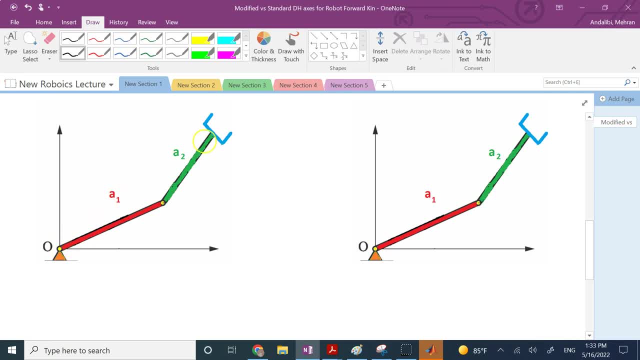 one and, if you remember, we named the joints from one to n, but the links from zero to n, and link zero is the base frame, is the ground, is the stationary one. so this is joint one. but the axis that i put on this joint one, if you call, if you recall, i would call it z, number zero, although this is joint. 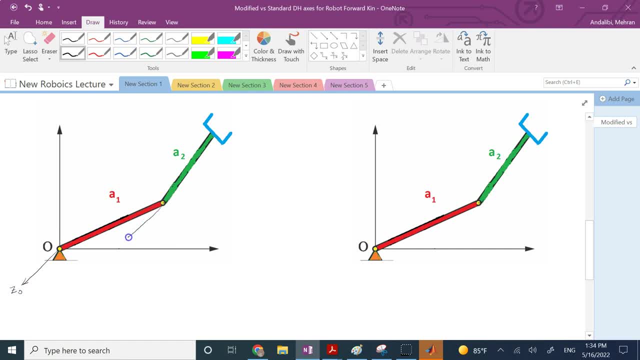 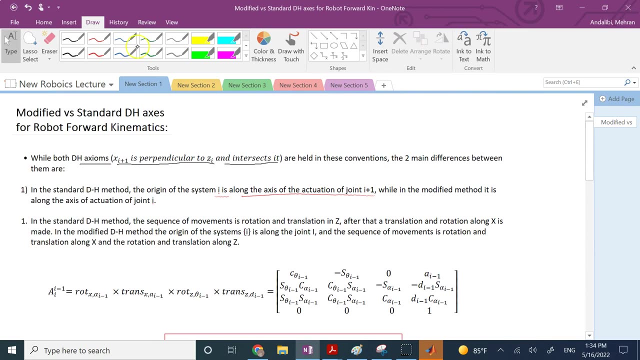 and this is joint two here, but i would call the actuation axis for that z what one? okay. so this is how we did, the standard or classic, but in the modified it's not the case here. if joint is i, then the actuation axis for that is also what is also z i, not z i minus one. okay, so basically. 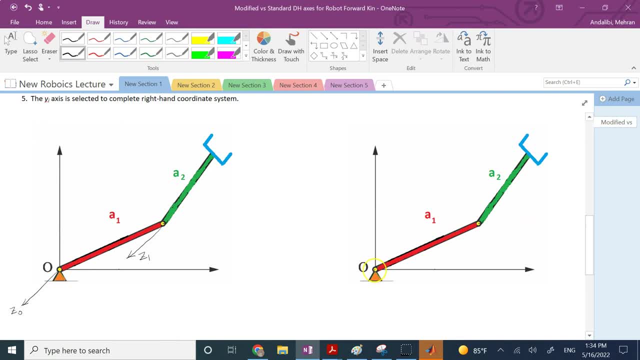 if this is joint number one here, then the actuation axis for this is also going to be called z1 and this is joint 2, so the actuation axis here is going to be called z number 2.. so that's one of the major differences between these two methods and that's kind of the advantage of hey, if this. 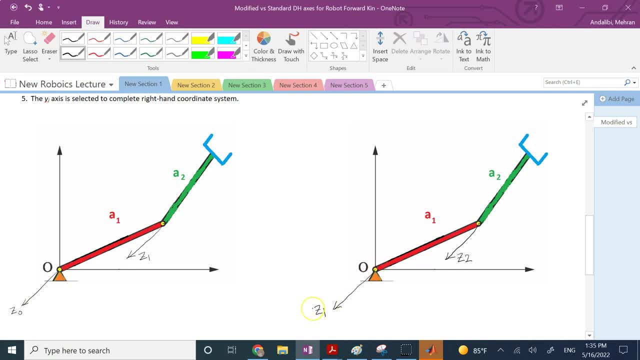 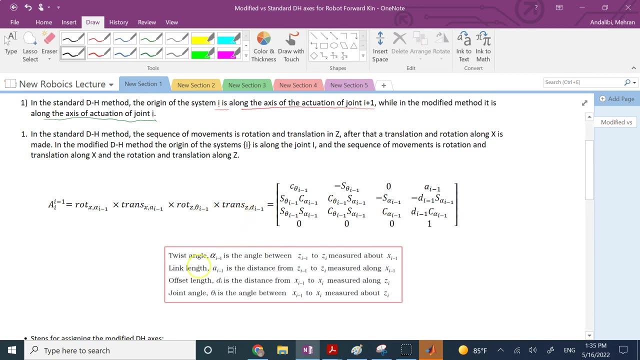 is joint one. i would rather the axis of it also be called z1 not z0, so it is a little bit more meaningful in that sense. but that's not the only thing. the other thing is the order that we use for translation and rotation, with these four parameters- a, d, alpha and theta- to go from one frame to the. 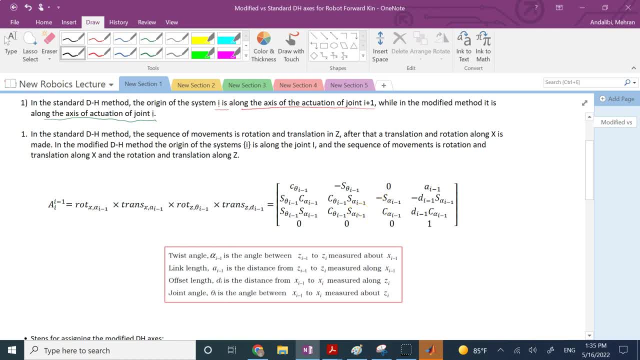 next, if you remember the order that we had in the classic um, the edge was what the a of i with respect to i minus 1. it was starting with a rotation about the z-axis, so it was a rotation of z and the angle was theta i multiplied by the rotation matrix. or translation, actually translation about. 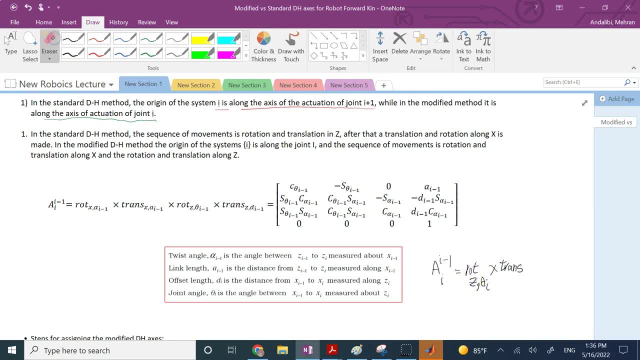 which z, the previous z. so if i want to call that z, give it an index. let's do that. it's more appropriate for the z. so this is z i minus 1, and the angle was also theta i minus 1.. then align that same z. 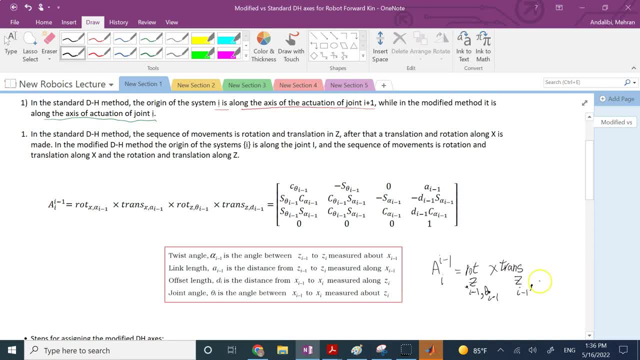 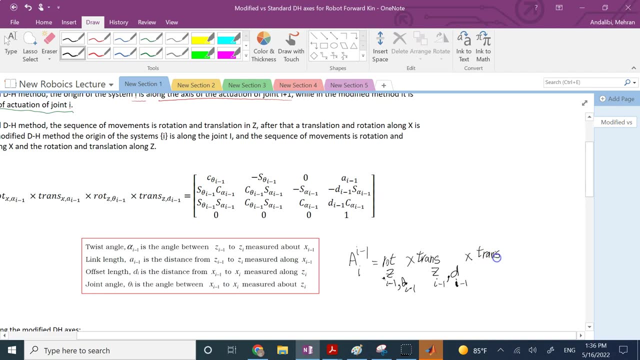 i would translate. for what? for the distance, d i minus 1.. so a rotation z, followed by a translation z, then followed by a translation about the new axis x, and the distance was a i minus 1, and finally followed by a rotation about the new x-axis, and. 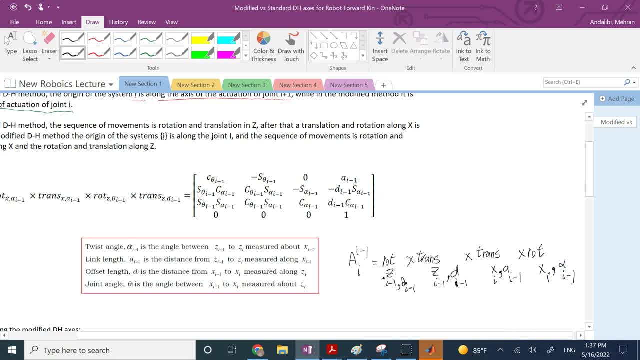 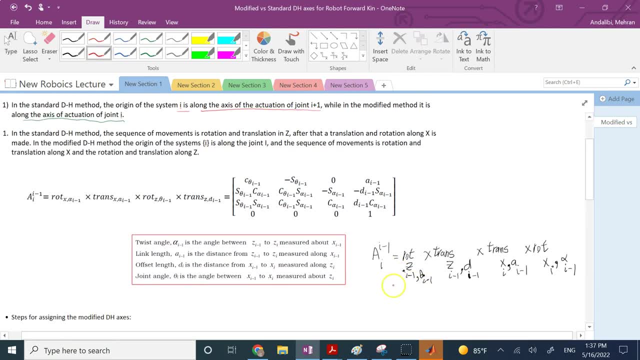 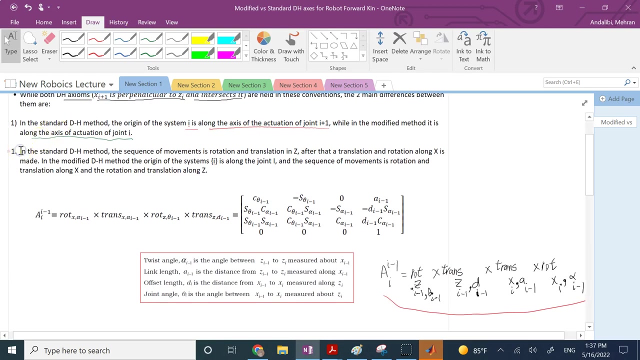 the twist angle. so this is the order right of the rotation z and the distance that we had in the classic d h or standard d h rotations- the translation z, translation x, rotation x, while here in the um uh, modified method, the order is a little bit different. what is the order here? it is rotation. 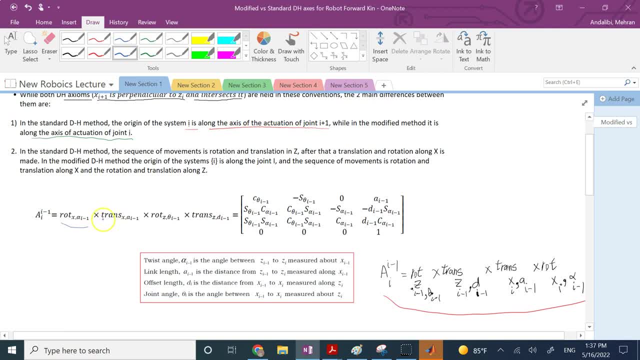 next of alpha, followed by translation x of a, followed by a rotation z of theta, followed by a translation of z and b. so first of all, you see, the x's come first, then the z's, and then the order is rotation translation, rotation translation. so the order is also reserved right. rotation translation, the next. 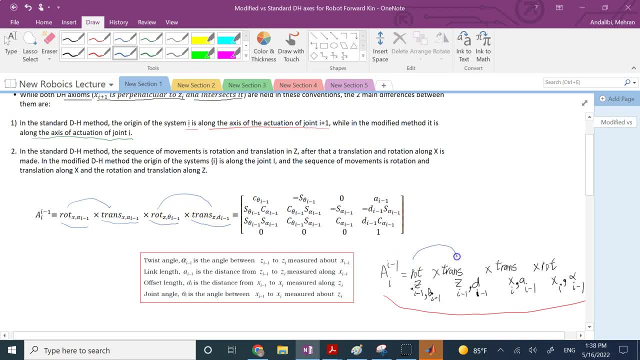 set is also rotation translation. well, here is rotation translation, but here is what translation rotation? so the order is reversed also as you go from z to x. so that might also be a little bit what easier to follow. that is rotation translation, rotation translation, not the other way around. 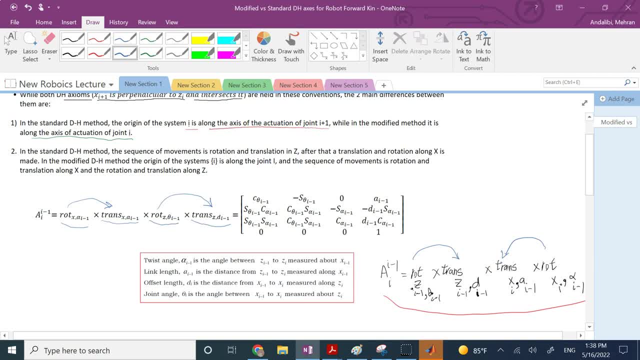 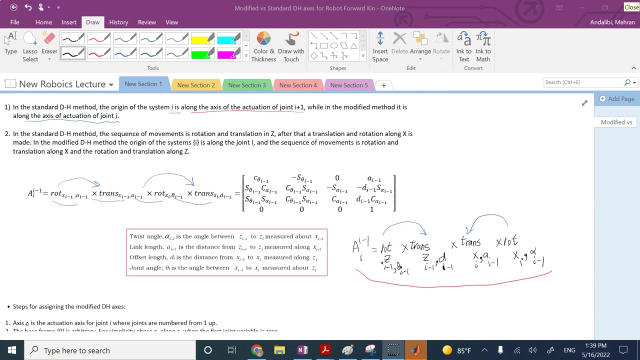 it's not a big advantage, but overall, you can see that this modified is really meant to make it easier to keep in mind and easier to follow. okay, but other than that, that's it really. that's all there is in terms of the difference between what the classic and the modified dh, and here i have added these, i minus ones and i's for. 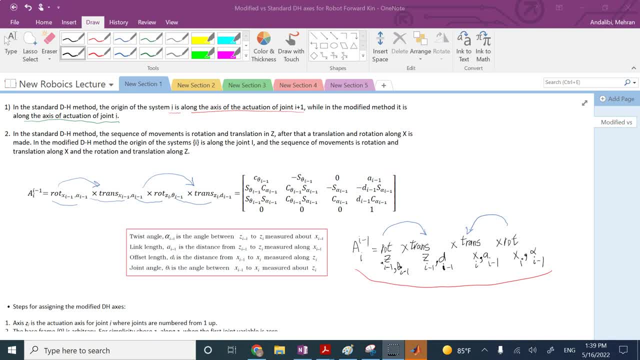 x and z axis as well, so you know exactly which axis is it. it's always the first two are the axes of the previous frame and the next two are always the axis of the new frame. okay, but which order in the modified, as i said, translation rotation, followed by another translator rotation rotation, translation and the. 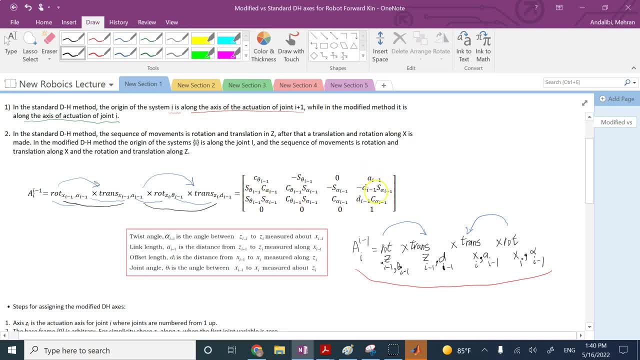 overall matrix, the overall homogeneous matrix of the dh is going to be this guy that you see: c theta negative s theta right, and then s theta s, theta, c, theta, c theta multiplied by c and s, of the alpha negative s alpha, c, alpha, a negative d times s alpha and d times c alpha, zero, zero one. so the last row is still zero, zero. 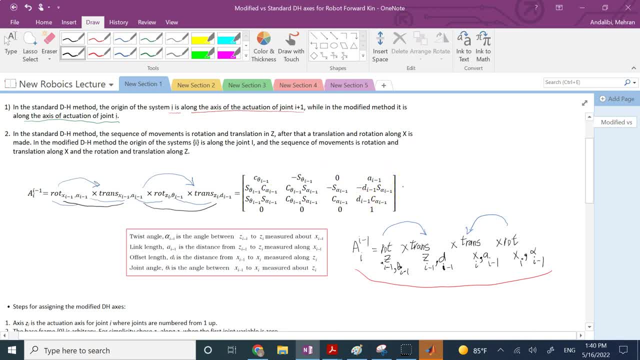 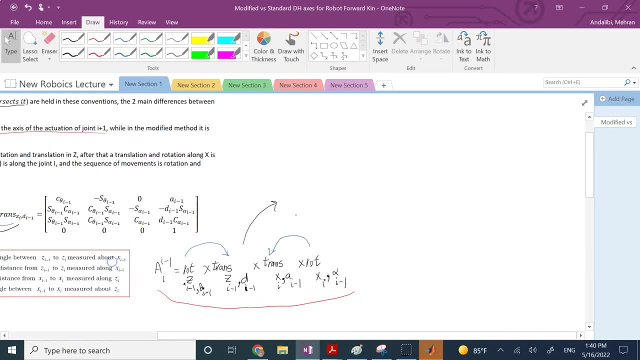 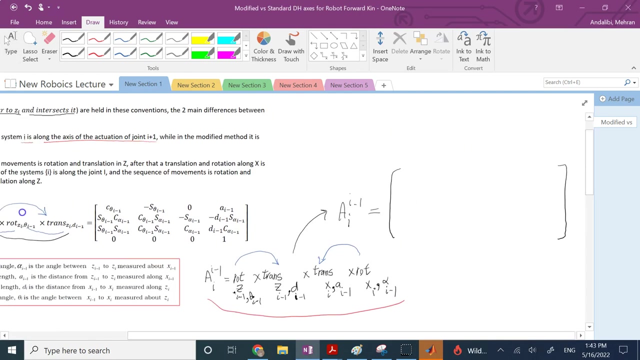 one, but the first three rows are clearly, what? clearly different. if you remember in the classic, the matrix that we had a of i in i minus one, or with respect to i minus one, uh, it was basically this matrix. okay, so the elements that we had, they were basically c of. 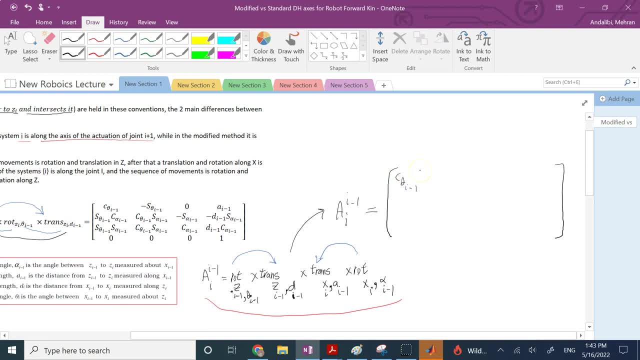 theta i minus one. and then we have negative s of theta i minus one times c of alpha i minus one. and then we had s of theta i minus one times s of alpha i minus 1. then we had a i minus one, c of theta i minus 1. this was s of theta i minus 1. 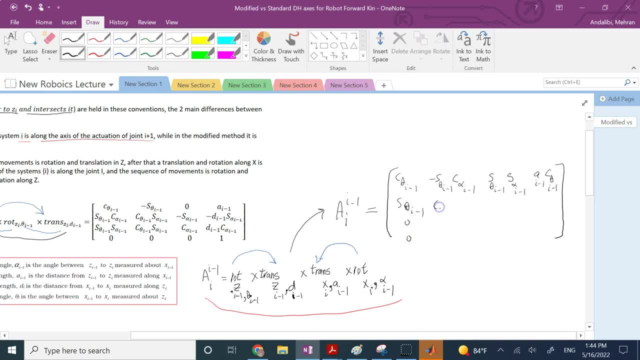 zero, zero. here you had c of theta i minus 1 times c of alpha, i minus 1, followed by negative c of theta times s of alpha. this was a of i minus 1 times s of theta i minus 1, and then d of i minus one and then a zero. this was 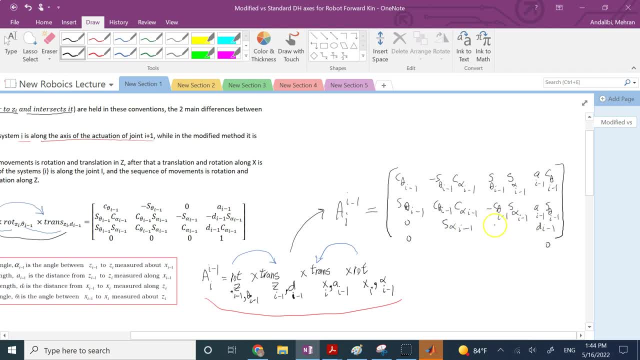 s of alpha minus one, this is c of alpha i minus one, and this is a one, not a zero, this is a one. so if you look at the difference between these two again, you clearly can see some real big differences, i would say, except for the last row and maybe the element one one. 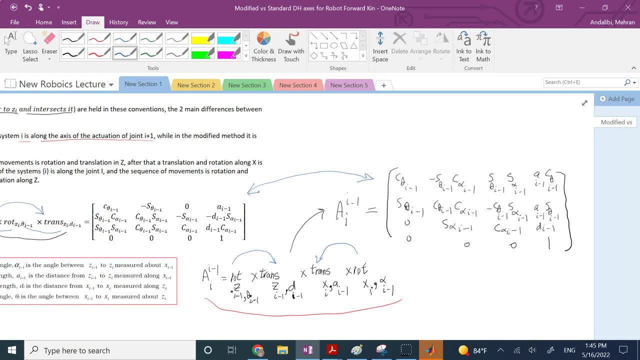 most of it is different, right like here. you see the d is repeated in two places, while here the a is repeated in, here it is repeated in the basically x and y of frame. i in i minus one, you have a. here in y and z you have d, and the reason that d here shows in. 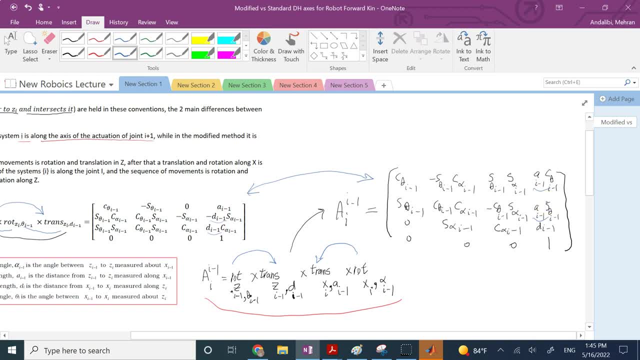 two places here. a shows in two places is because the order is reversed. right here. d comes basically, if you look at it, last. so it is already affected by alpha and everything. here a is the one that comes second to last. okay, so because that order is different. 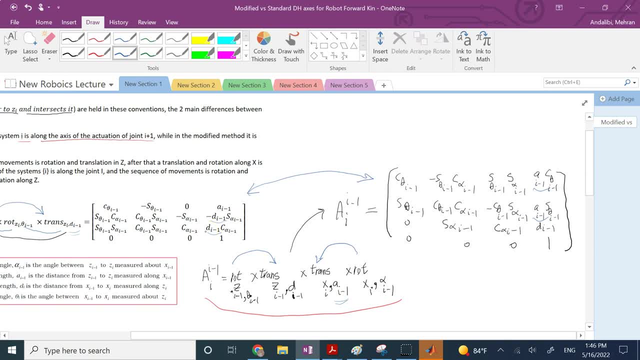 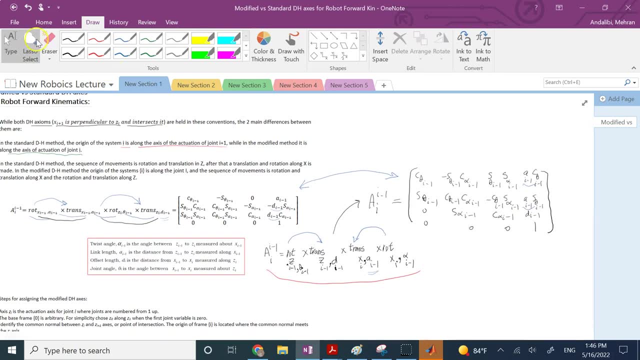 the transformation homogenous transformation matrix is quite a bit different and again here i can put them for you side by side. if you want to see everything in one place, i can put it all for you side by side so you can see the difference, right? so these two 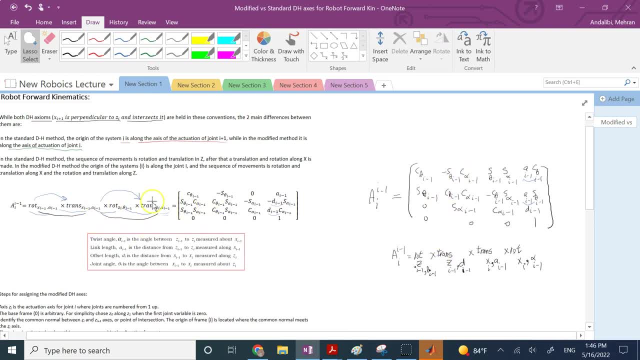 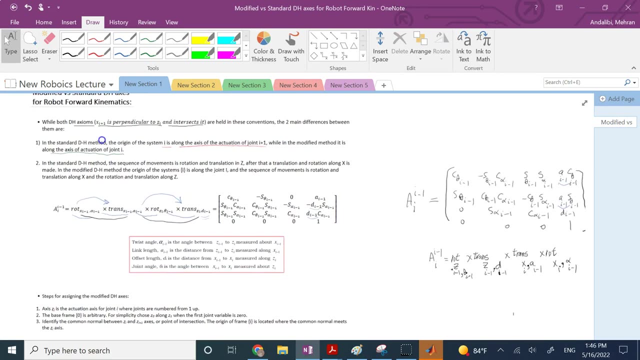 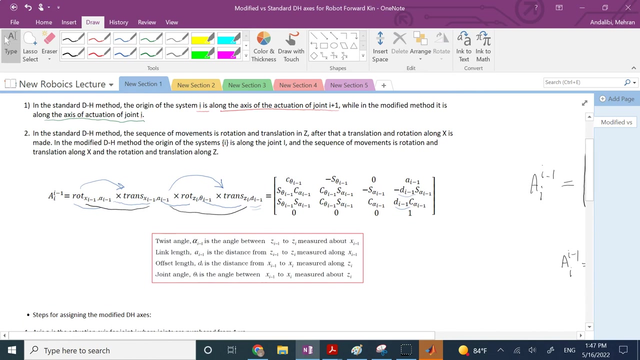 are for classic, and then this guy here on the left is for modified, or you can come and combine those two into one big equation like this. okay, so this is the main difference between these two conventions, now going and focusing on the modified frame, because we already covered the standard, so we're going to solve a couple. 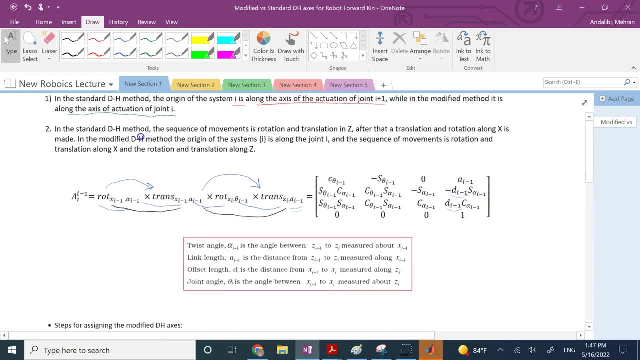 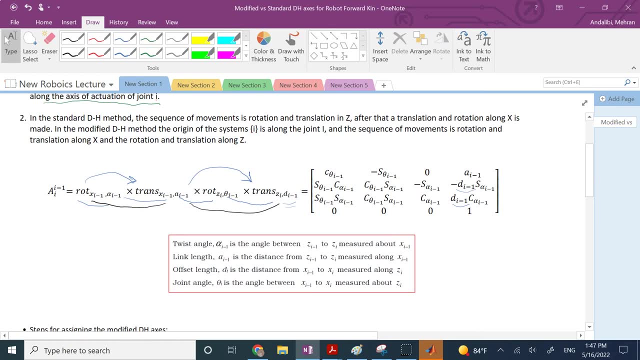 of examples on the modified frame really here. so the definitions of alpha, a, d and theta are provided to you here. so alpha is still the angle between z, i minus one and z. right, it was the same. alpha was the angle between the z's. still the angle between the. 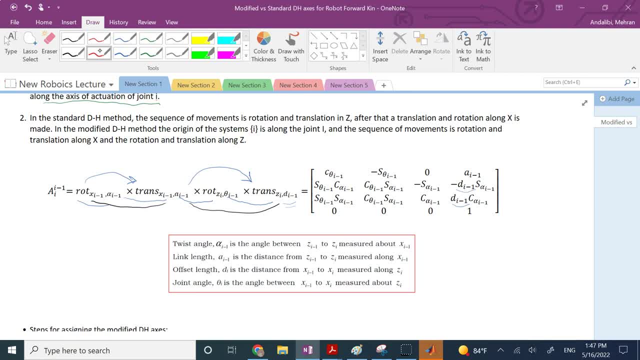 z's, but in the standard one it was about the axis xi. here is xi minus one, because it comes first, and a is also the distance between z, i minus one and z allowing x, but this x is now the previous x. on the other hand, the two things that were about the old z in the classic 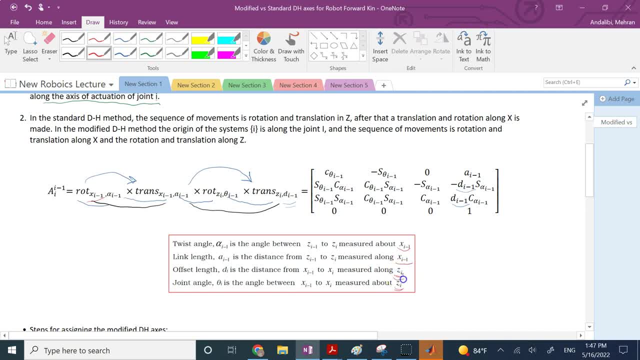 now they are about the new z. what are they? they are what? the angle between x i n i minus 1 and x, which we call theta i, and the offset between x i minus 1 and x aligned z i, which we called d i. okay, so, uh, basically, you see, it's just a change of order that is happening here. 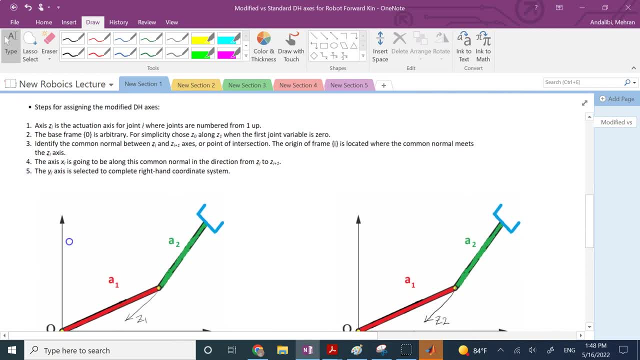 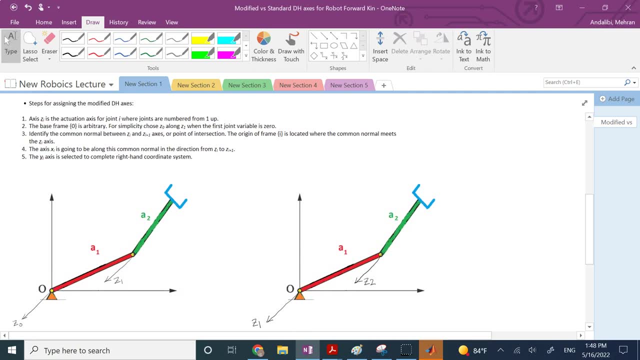 so now we want, with basically accompanying examples, we want to talk about what- setting up the frames, with two examples of the modified frame and at the same time i also, just to refresh your mind, show the axis for what? for the classic one as well, for the same robot. 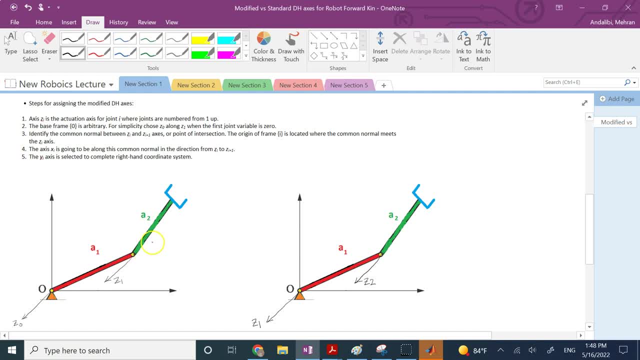 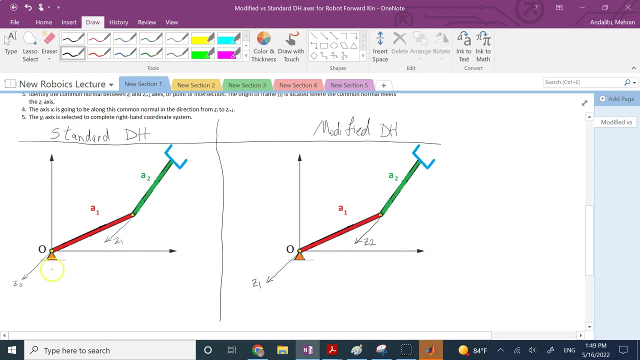 so again, side by side, you can see the difference. so here on the left i'm going to do basically the standard dh, while here i'm going to do modify the edge, okay, so let's see what we have. so in the standard it was clear the actuation axis for joint i 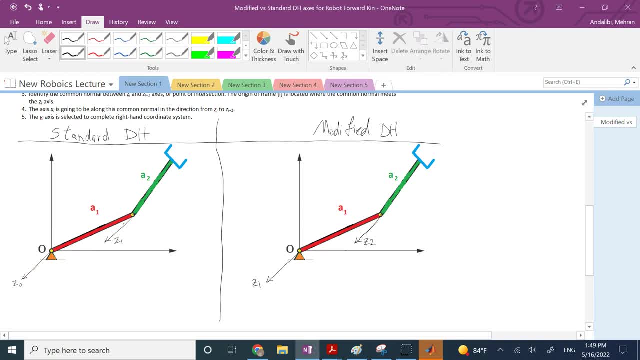 is z i minus 1, so z 0 and z 1 clearly defined. and here i choose these two axes to be my x not and y not. as you know, the origin and the orientation of x and y are arbitrary, so i just choose them the way that you can see. and then now x 1. here x 1 should be intersecting and perpendicular to 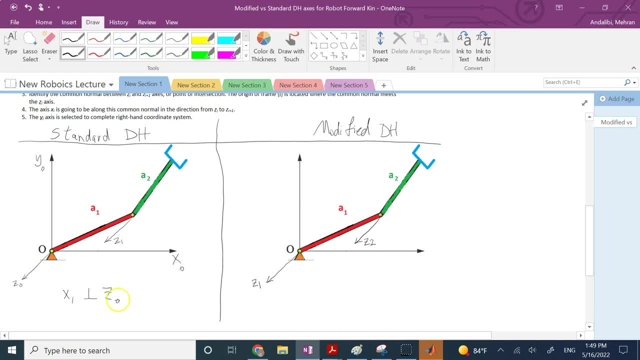 zero. x i should be perpendicular and intersecting, z i minus one, so x one should be intersecting and perpendicular to z zero. and here z zero and z one are parallel, so any normal to both would work. so here i choose the axis along this red member, the first member, and i call this x one. 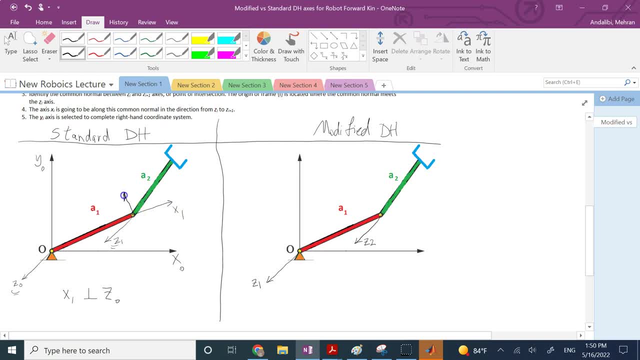 and y axis is always determined by the right hand rule, so that is going to be y1, and here we also need an end effector frame. and for the end effector frame i choose my z, in this case to be out of the board, like z zero and z one to minimize the number of required. 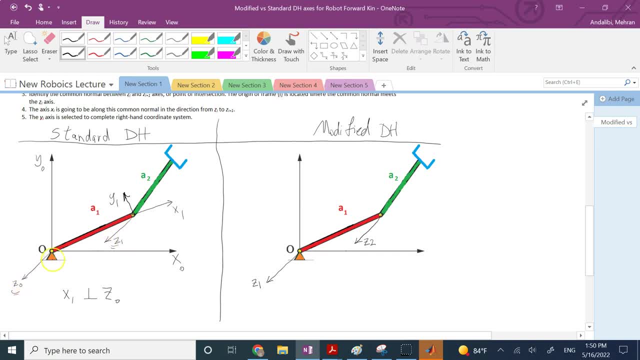 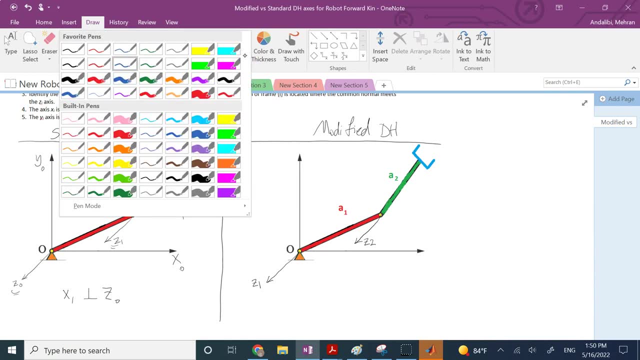 parameters that are non-zero. so, by the way, this z zero and z one are out of the board, making a z zero is a non-zero and z one is a non-zero and z one is a non-zero and z one is a non-zero. maybe here i use a separate color to indicate them for you that these two frame these, whatever. 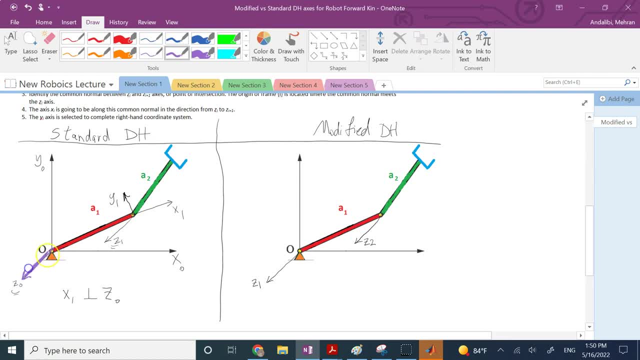 i hear, use a black, a purple color, for whatever i use a purple color, that frame is out of the board, okay, or i can show the sign of out of the board which is like this: right, i can do that one as well. so, um, here this is going to be my z number. 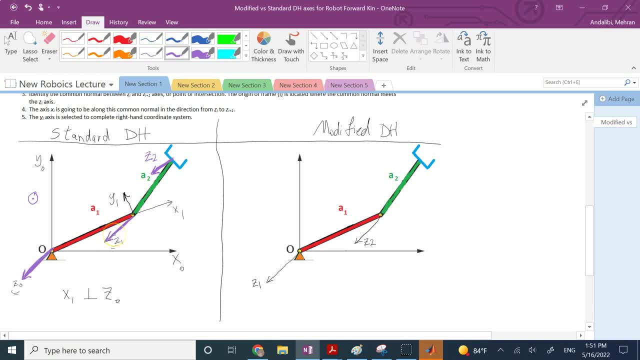 two. again, i choose it to be the same as z1 to minimize the number of non-zero parameters. and now x2 should also be perpendicular to z1. again, z1 and z2 are parallel. any common normal would work, and so i choose my x2 to be allowing the green member like this: 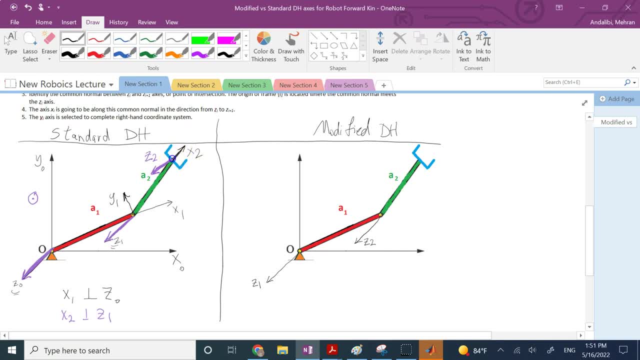 and that's means your y2 is going to be perpendicular like that. okay, so that is y2, and so this is z number two. good, so this is what we had, if you remember, for the uh standard gauge. now, if we look at the modified one, the axis, actuation axis of joint one is z1. the actuation axis for joint two is z2. right, 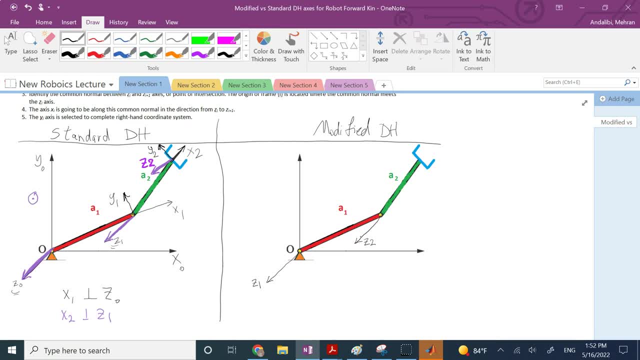 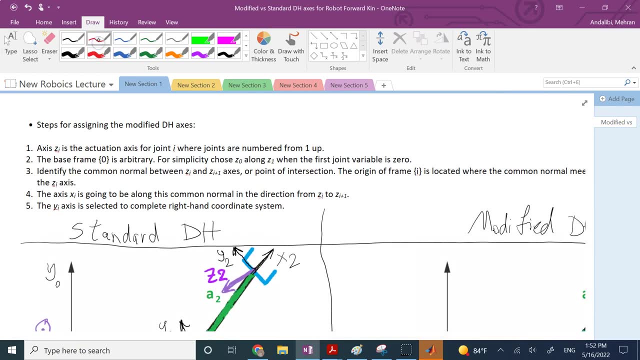 so you might say, well, where would you put z0 now? well, z0 is arbitrary. one suggestion that i provided to you here is: if you want a simple solution is to choose z0 and z1 to basically be on the top of each other. okay, that makes life easier. it minimizes the number of 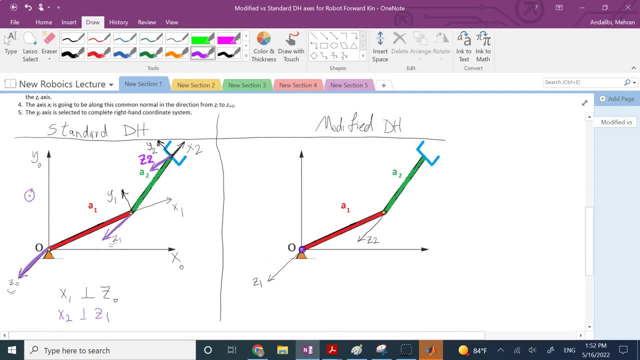 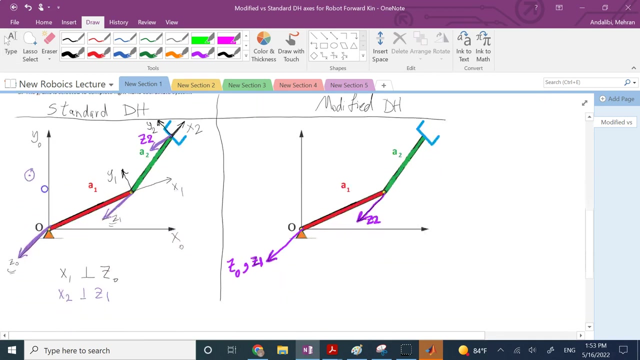 parameters that you need. so in this case, of course, just like the previous case- z1 and z2, which are out of the board- i say i choose my z naught to be the same as z1, to make it as simple as possible. good then, what well, you can choose also x0 and y. 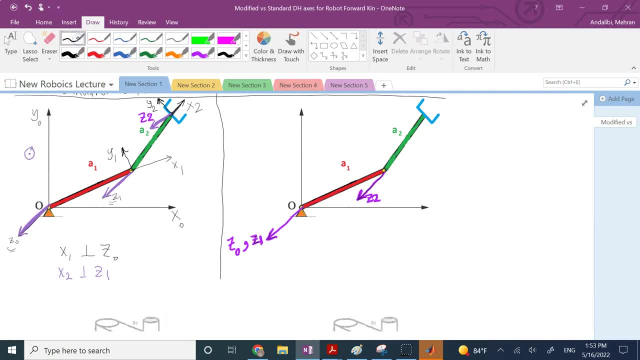 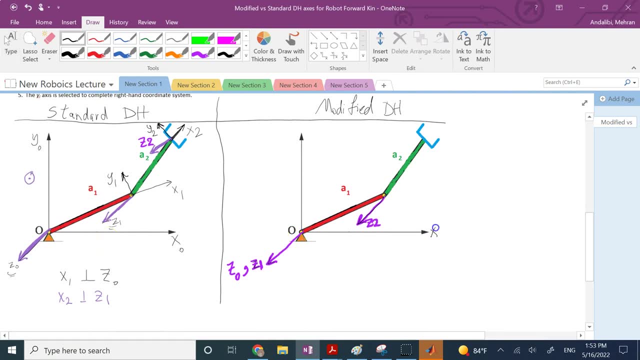 zero and the origin of this frame arbitrarily, so i try to make it as simple as possible and as similar as possible to the standard. so i choose this one to be x naught and this one to be y naught and origin to be a joint one right now. 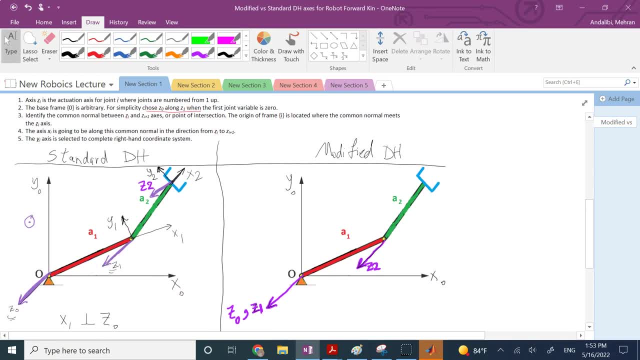 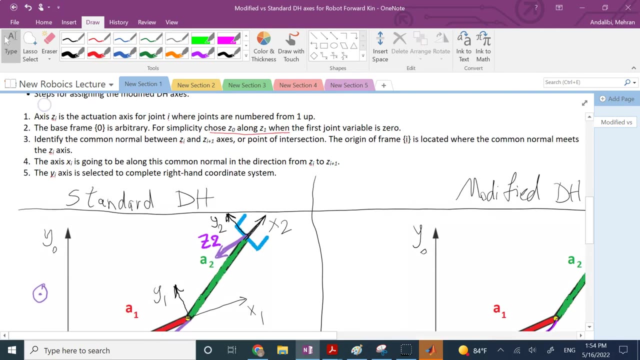 the next step is this: now you want x of frame one, you need what x of frame one and the origin of frame one. and this is where this lines three and four would come to help you. and they say: find the common normal between z i and z i, plus one that is going to have the common nor. 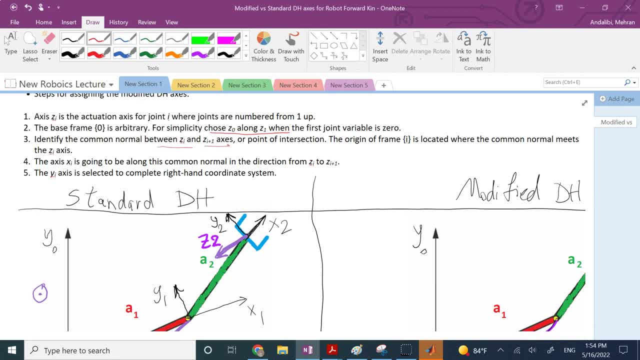 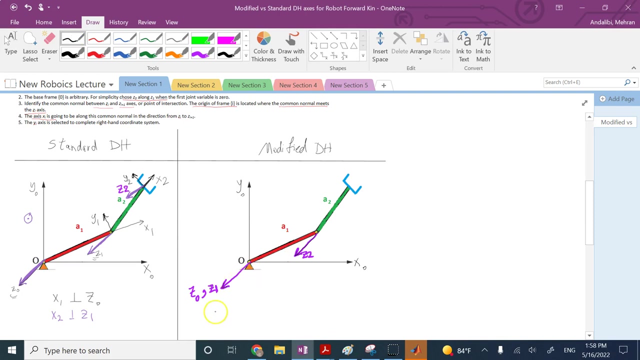 normal that is going to first of all align. this common normal is going to be your x of i and your origin of frame i is also located where this common normal will intersect or meet z i. so now, if you want to apply it for this robot and if you use i, equal one right, we want to get to x and i, so 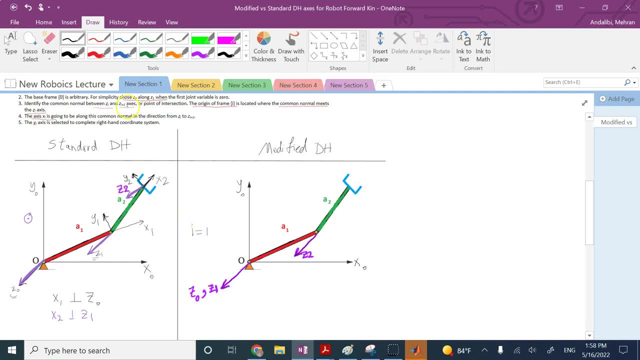 here is the x advice of this common normal. alright, i equal one and apply this. uh, parts three and four. it says: uh, you look at z1 and z2. right, they have a common normal. in this case they are basically parallel. so they have infinitely many normals. you can choose one of them and i would choose basically the one that is on the x, not y. 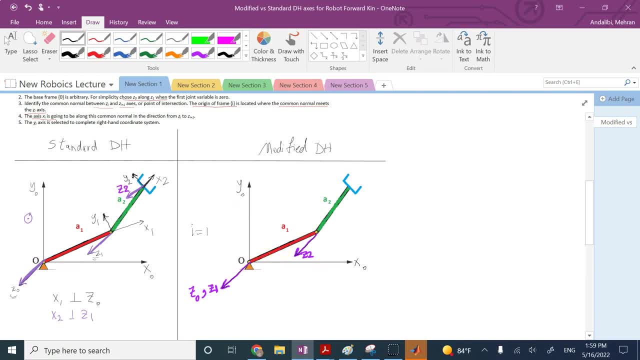 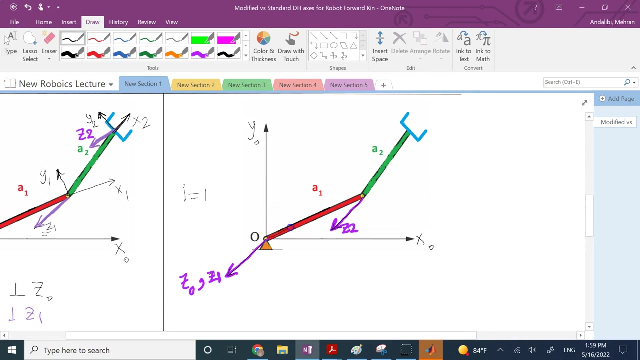 not plane along the red member. that is going to be perpendicular to both and, uh, that is going to be the direction for your xi. and wherever it that xi will intersect, the axis z1, that's x1, is going to be, of course, origin one. so this is clearly that common normal that i want, this common normal here. 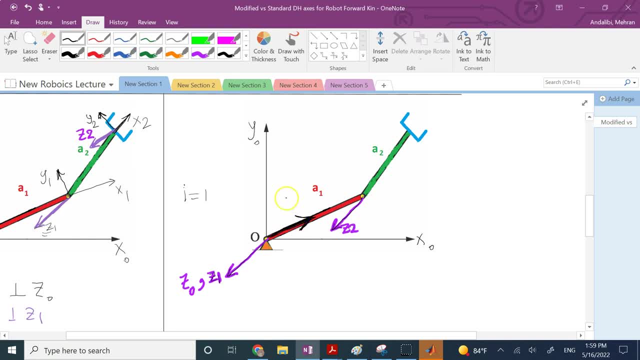 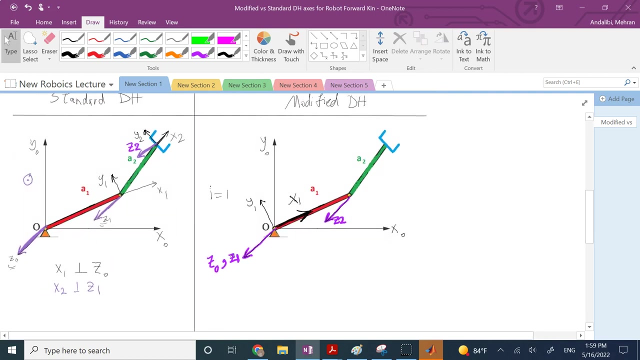 right that i would call x1, and of course it is going to cut z1 at joint number one, and so my uh y axis is now also determined in the right uh based on the right hand system. so that's x1 and y1, and clearly, you see, x1 is similar to the previous case, with the difference that 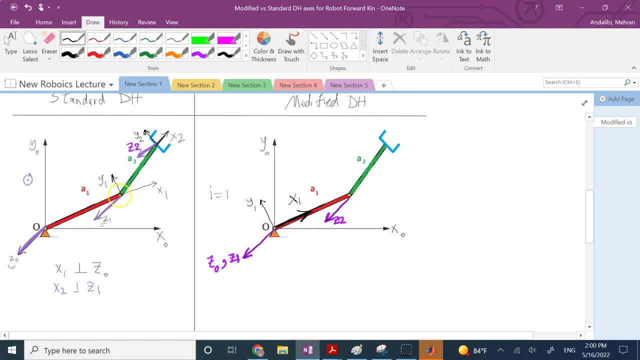 the origin of frame 1 is now a joint 1. in the previous case it was at joint two and that's what makes this modified dh to make more sense, because each origin and each frame is located at the corresponding joint, not one joint ahead of it. 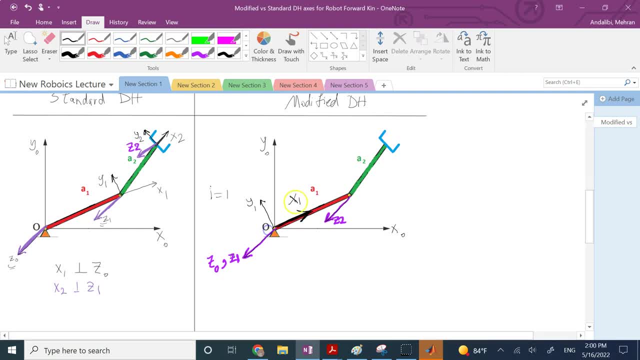 so now, uh, that's frame one, it's set up. now we go to i of two and repeat the same process. now, when we want to go to i of two, we have to look at z2 and z3. there is no z3 here. okay, there is no z3, so we can determine what x3 and origin- sorry, x2 and origin 2, right? 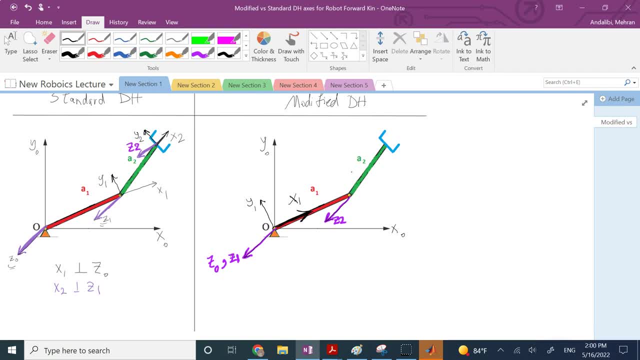 so we really need a z3 if we want to apply that rule, or we can just go with an arbitrary direction, like this in the previous case, and make x2 align the green member. but even if we do so and say, well, let's say x2 is aligned, this member, y2 is perpendicular. if we do that, then when we set up the dh table. 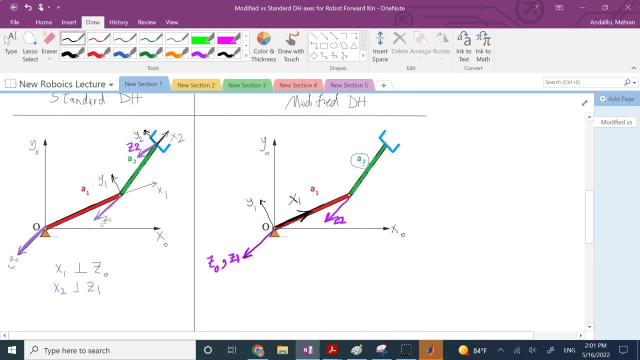 this parameter a2, will never be taken into consideration, because you are going to get something like this. so, and then, between frames zero and one, the only parameter that you would have involved is the first, angle, theta one, and that's it. between frames one and two, you will have angle theta two and 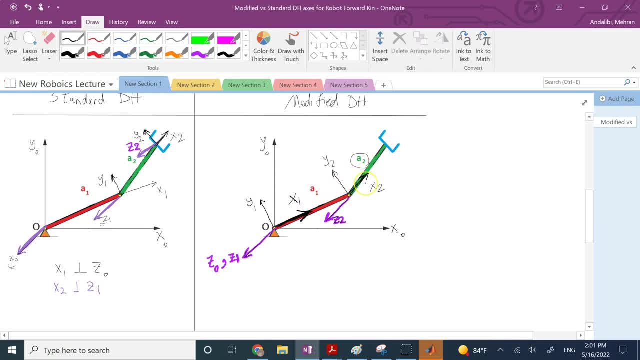 a1 and then a2, will never be included in your forward kinematics unless, as i said, you define a frame three here in the modified, so you can involve the angle at the distance, a2, or the length, length, length, a 2. okay, so, uh, that's where in the modified frame, in this scenario, we need an extra. 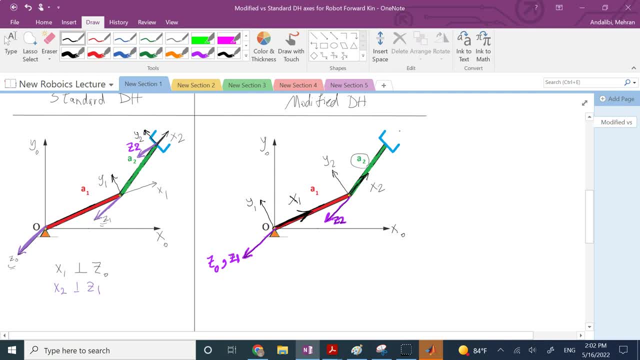 frame. okay, we need an extra z3 and that is really going to be for the gripper right now. so where would you put the z of that gripper? again, it is um, in this case i try to go and it's not uh, but it did work pretty well. so i would uh invest some time on this to see if that will work. 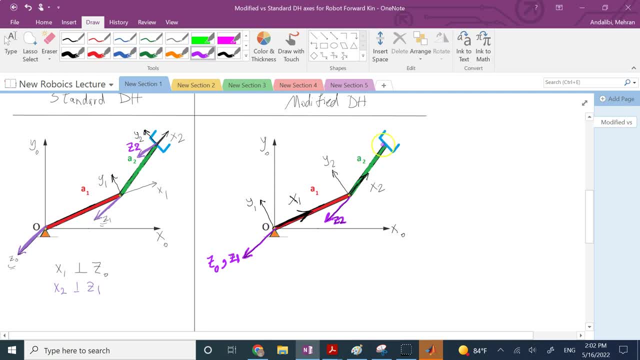 you really want to be shooting this at a y2 f where- and what i mean by that is that your length, length in that's, this is very, very important now. um, so in vitus we you really want to kind of move the feeding out of the board to minimize the number of non-zero parameters. so i say that is for me z number three. 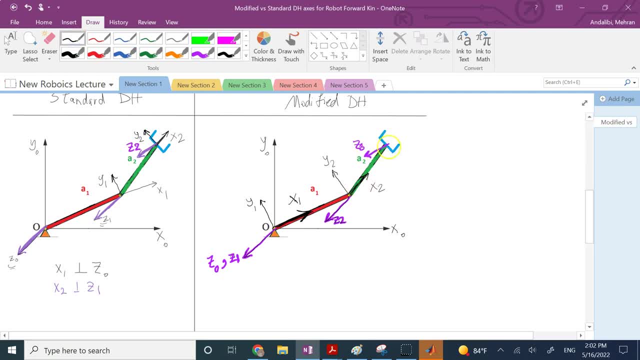 and if that's the case, now again, i have infinitely many normals between z2 and z3. this x2 is a good one, so i choose that x2. that's origin 2.. now what about x3 and y3? well, for x3 there is. 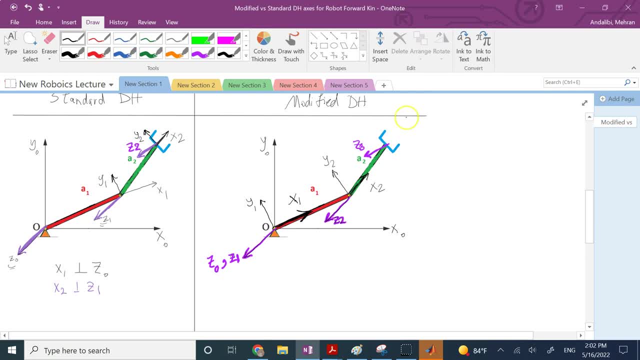 definitely no new z. there is no z4, so for x3 here i'm free to choose, and since i want to minimize the number of parameters- in this case theta, which is the rotation between one x and the next x along z, i try to lock that frame three to this member. so i choose x3 to exactly be the same as x2. this 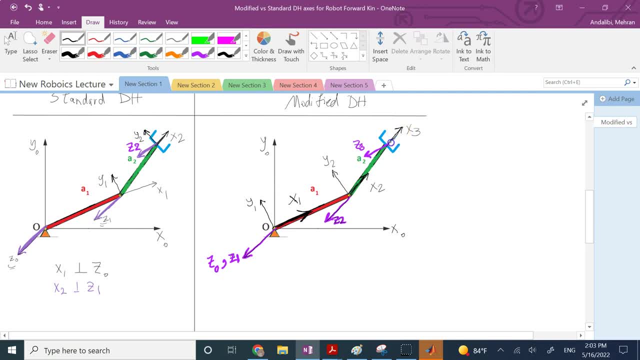 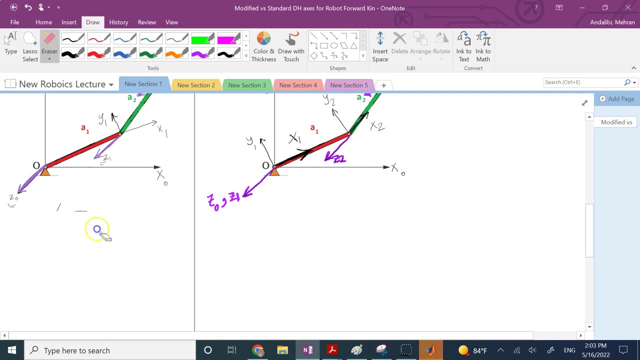 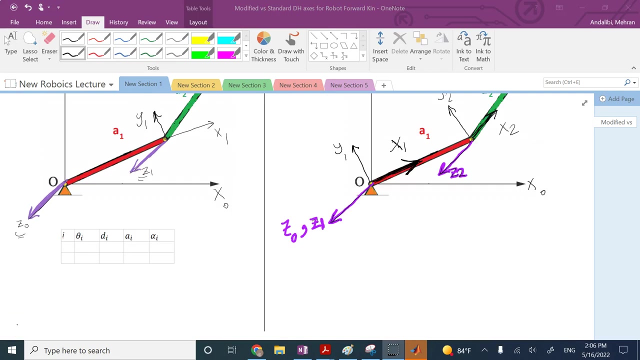 way, the parameter theta between two and three will be zero, zero, and so this is going to be your y number three. okay, so now if i want to show you the ds table, right, let's see how we can fill it. so this is the dhx table for um, the um. 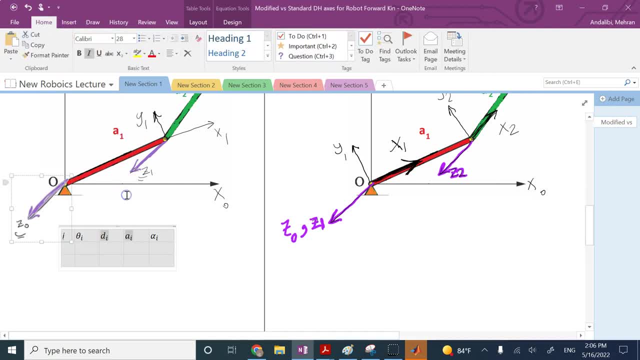 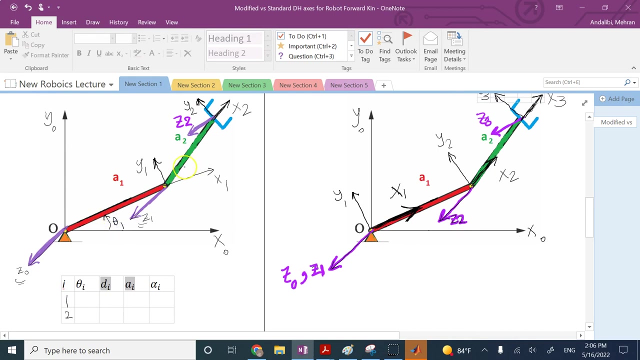 standard system. right, and let's see if i can make them a little bit bigger. right, there we go. so here what we have is one and two and the angle, because you know this angle is going to be theta one and this angle here is theta 2.. so you will have theta 1 will become theta 1. 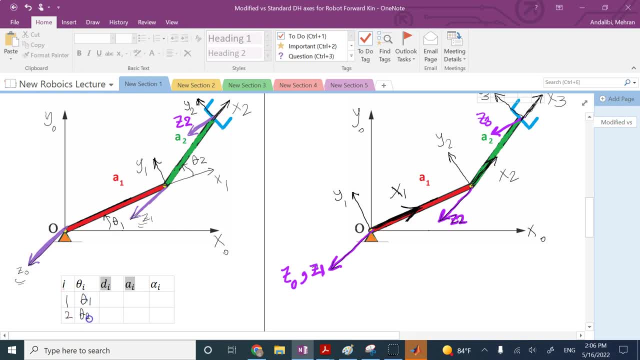 so you will have theta 1, one and theta two, and these are the variables, right with respect to time and um. then these are the displacements along the old z, since these are out of the plane. nothing moves out of the plane as you go from one joint to the next or one frame to the next. 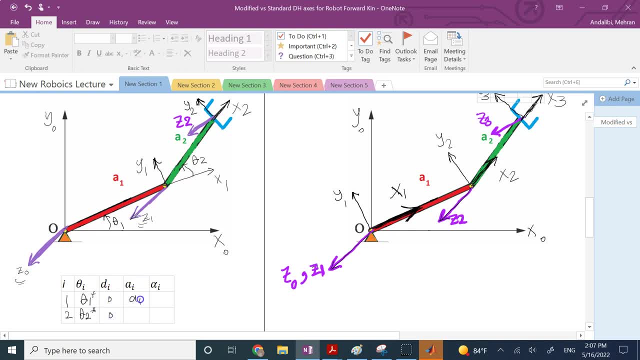 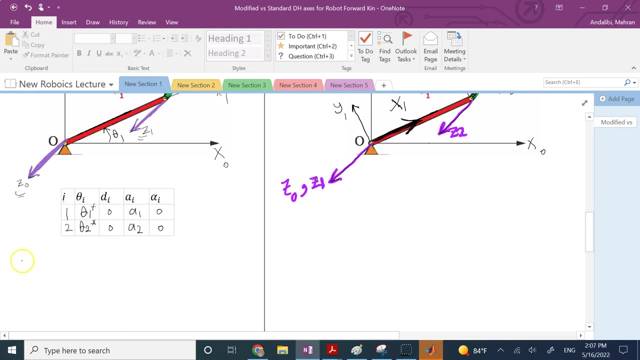 these are both zero, a's are a1 and a2 and in this case, again, all these are align, so there is no twist. okay, so that is your dh table and if you calculate your final uh t matrix, t of 2 with respect to 0, which is a of basically 1 with respect to 0 times a of 2 with respect to: 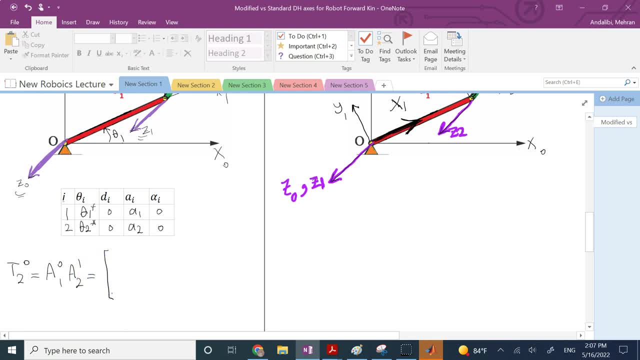 to one, the total transformation matrix. as you know, this is going to be c one two, negative, s one two, s one two, c one, two, and then you have zero, zero, zero, zero one. so this is a rotation z matrix with angle one plus two. the last row is always zero zero one, and here you will have basically a1, c1. 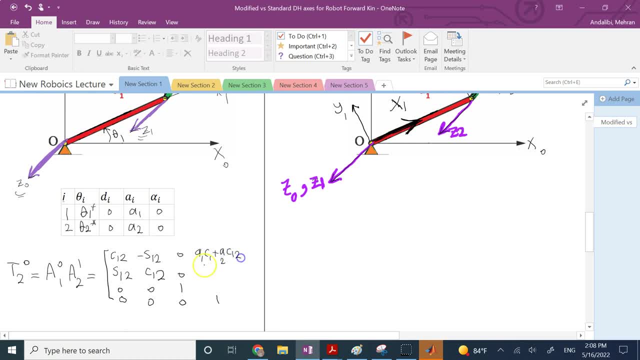 plus a2, c12, a1, s1 plus a2, s12 and zero. and you know, c12 and s12 is the sine cosine and sine of angle. one plus two, theta, one plus theta two, right, so this is what we have and clearly this part is. 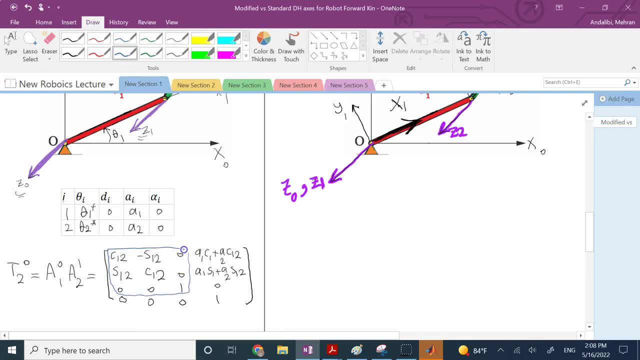 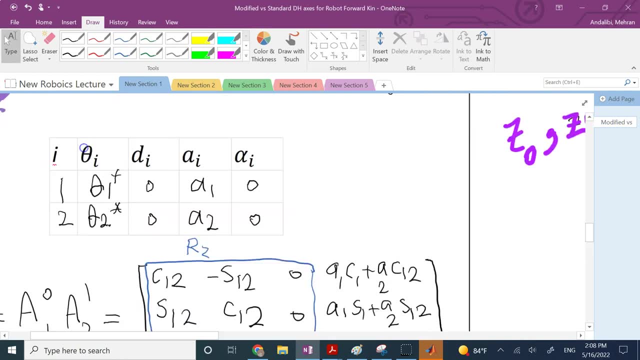 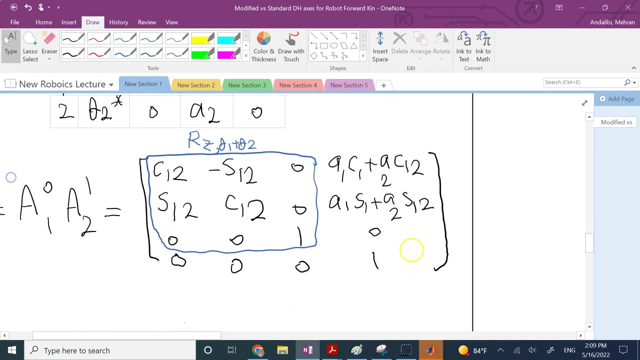 the rotation matrix, which is the rotation of z angle, theta one plus theta two. correct? let me see if i can write it bigger. and these are the x, y and z, z of the end effector in base. this is r of end effector in base, or r of two if you want. 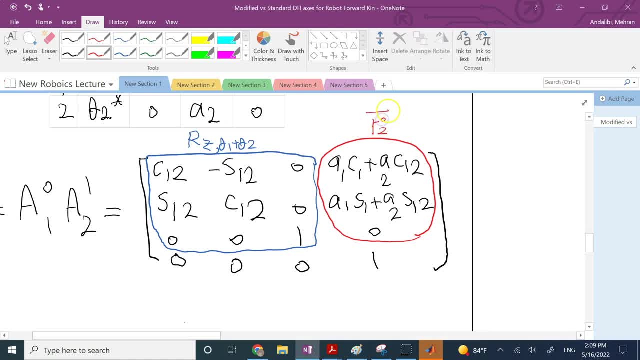 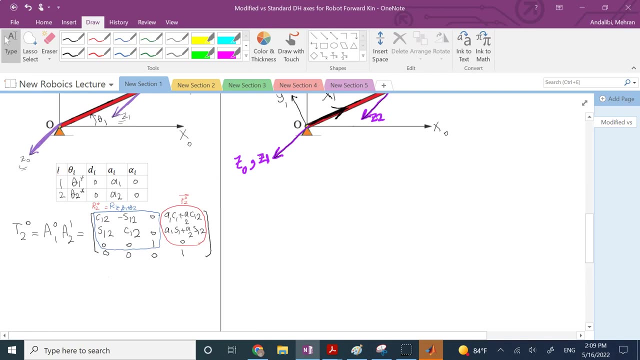 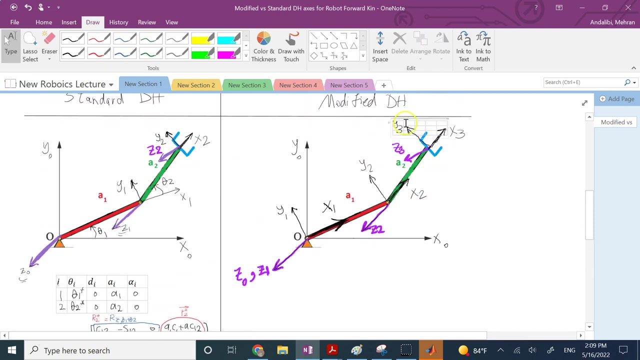 you might call it r of two in zero. right, this is the rotation of two in zero. so we have done this. now, if we want to do the dh table and the overall uh transform matrix from for the modified first of all, we have in this case uh three, three uh frames plus frame. 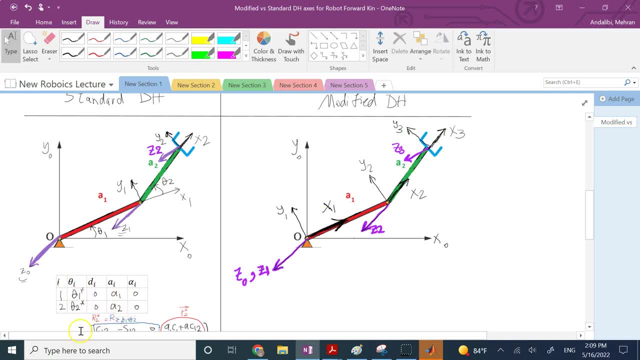 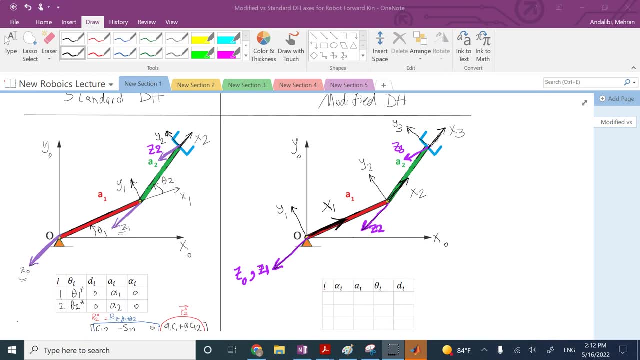 zero, so you will have three rows instead of two in your dh table. so, as i said, we have three rows here because we have overall four frames. i goes one, two and three here and um, the order is alpha a and z is also zero and d is awesome now. now i will show you another example of the alpha dB. 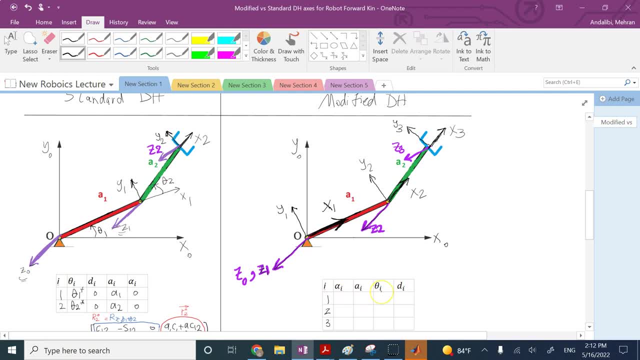 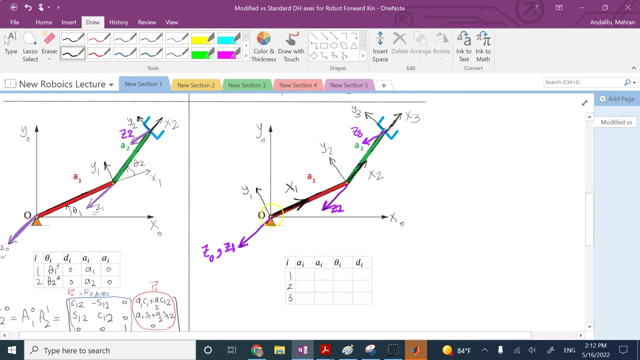 so if you look at the back of my slide here, we have said that whenever you are doing the axis, this is the x y, y. so you can see that I have done the x real angle that you have is this angle here, that is going from X 0 to X 1 and 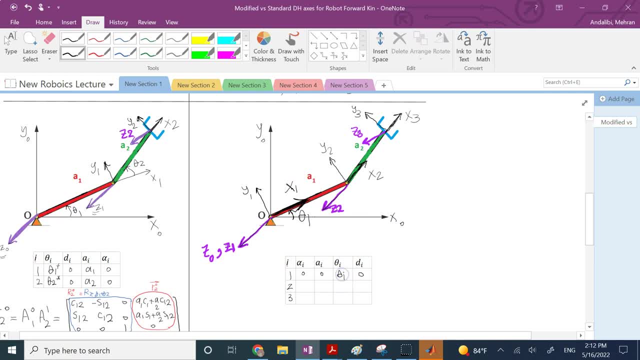 that is your angle, theta 1. so this is going to be theta 1, which is your joint variable. and then when you go from 1 to 2, now clearly the X's have a rotation angle. that is needed, right so clearly, if you extend this line, right like that. 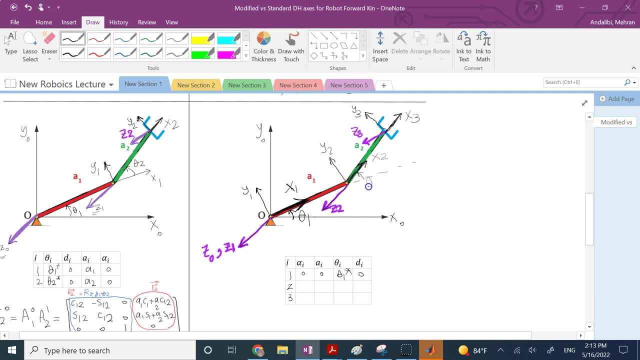 then you have this angle, which is theta number two that you need. so that goes here and then that's also the variable. if you can see no motion allowing, any Z is needed. origin 1 and 2 are on the same plane. no out of plane motion is needed. 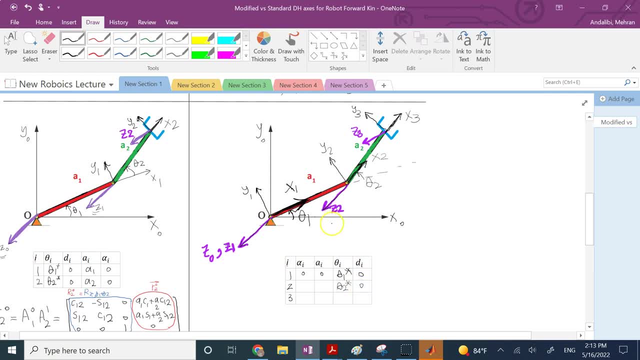 so no D is needed, and then align the old X, which is X 1. you need the translation of a 1, so this is going to be a 1. is there a twist needed? no, Z 1 and Z 2 are well aligned, so that is 0. then, as I go from 2 to 3, the Z's are already aligned again, so no. 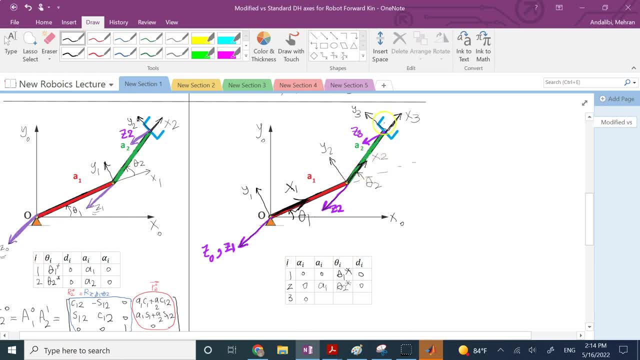 twist is needed. do I need to move, align the old X X 2? yes, that distance is a 2. do I need any rotation between them? no, if you remember, X 2 and X 3 are solidly attached to this member in green and the end effector is a solid attached to the. 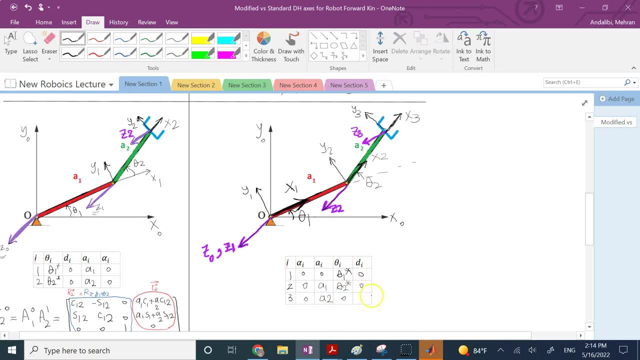 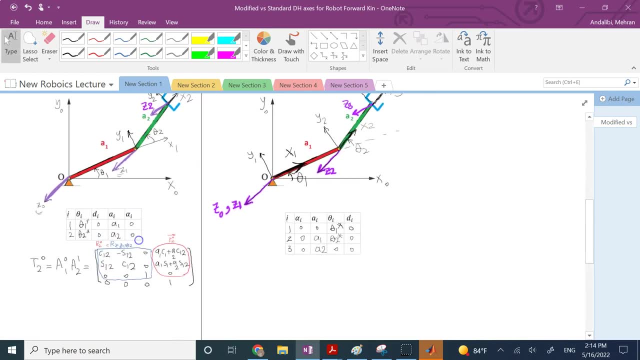 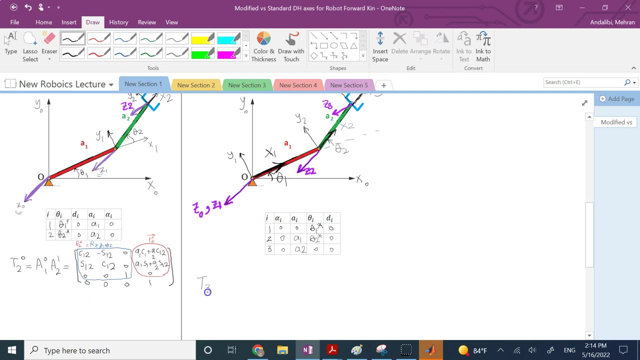 green member. so this angle is 0 and of course, no out of motion, out of plane motion, is needed. so D is 0. okay, and in this case, if you want the matrix, this is going to be T of 3 in 1 and this is going to be a of 1 in 0 times a of 2 in 1, times a of 3 in 2. and if you do that, 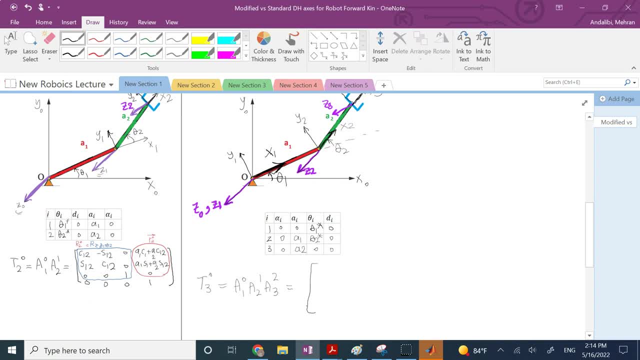 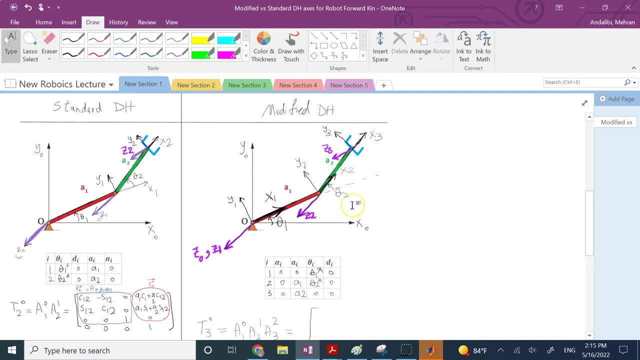 the interesting part is the solution will be what? what's your guess, do you think? because we talked about it, that's the transformation matrix looks quite a bit different. right, because the order is the same and that's why you look like the information is different. so let me make sure that that's. 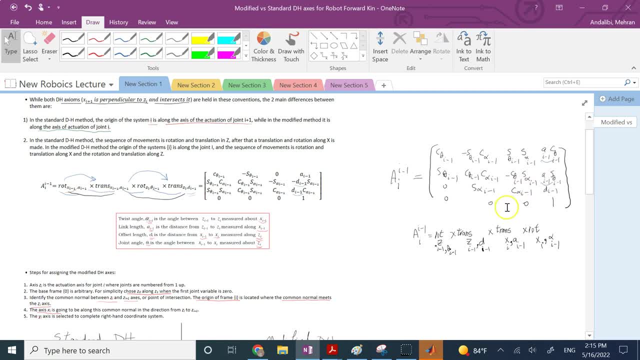 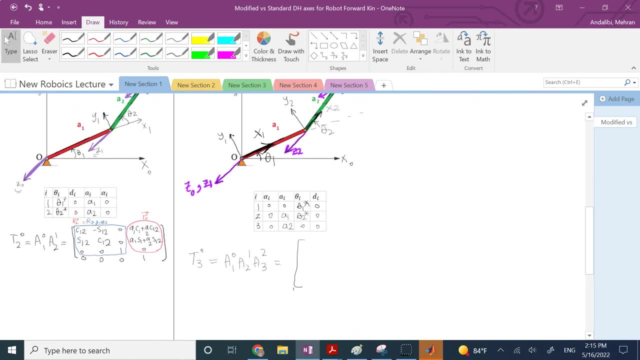 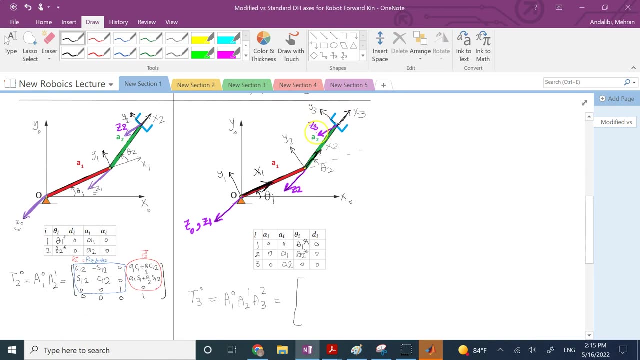 not true. yeah, and that's true, because the information in the matrix, in the matrix is is different. but if i go ahead and multiply everything together, right, what would you think? well, remember that if you look at the end frame, x, 3, y, 3 z 3, that's the same as x, 2, y, 2 z 2 of the 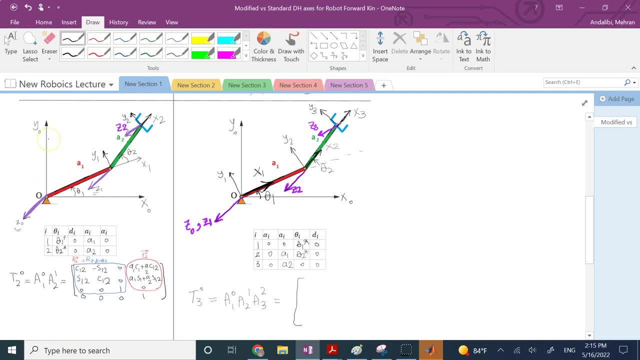 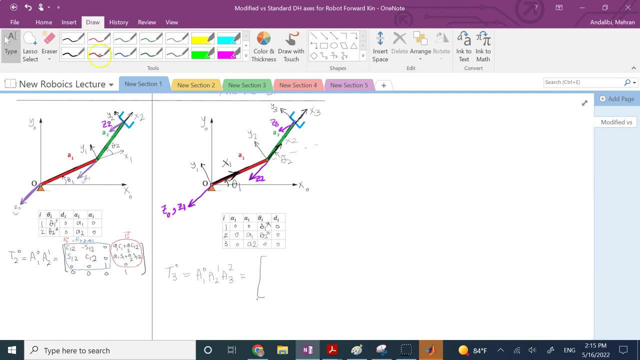 classic. they are the same thing and if you look at the frame zeros of them, that's also the same right. so the frame zero and three, the beginning and the end frame in both cases are the same. in this case, we call them three and zero. in this case, on the left, we call them two and zero. 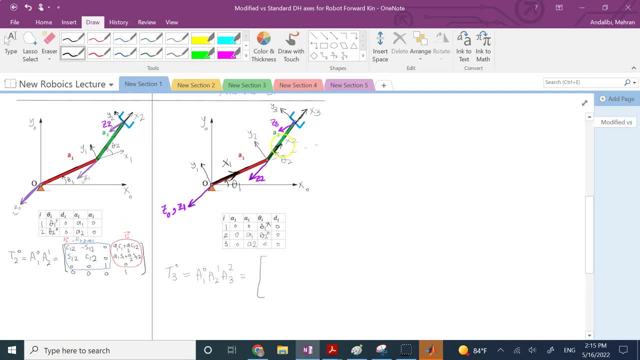 but they are the same thing, so whatever happens in between should have no effect whatsoever on this final result. so yes, if you do it, you will get c one, two negative s one, two, s one, two, c one, two, zero, zero, one, zero, zero, zero, zero, zero one, and then a one, c one plus a two, c one, two. 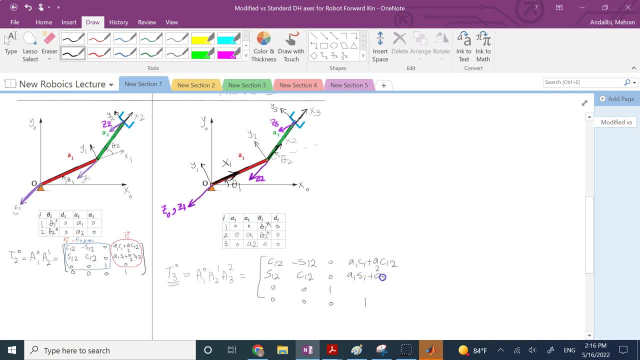 a one s one plus a two s one, two and zero. there is no difference. remember, you are describing the end frame with respect to beginning and as long as these two are the same and the parameters are the same, theta one and two, the definitions are the same: a one and a two, the definitions are the same. you should see no difference, although the 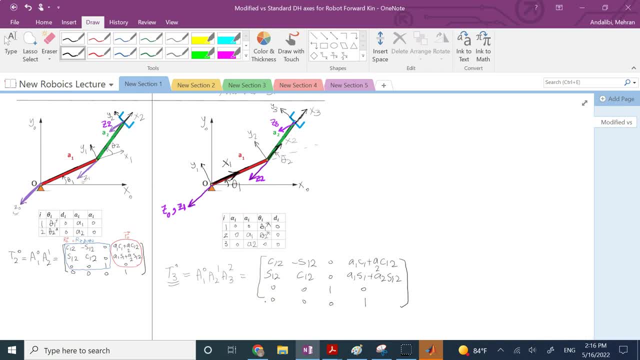 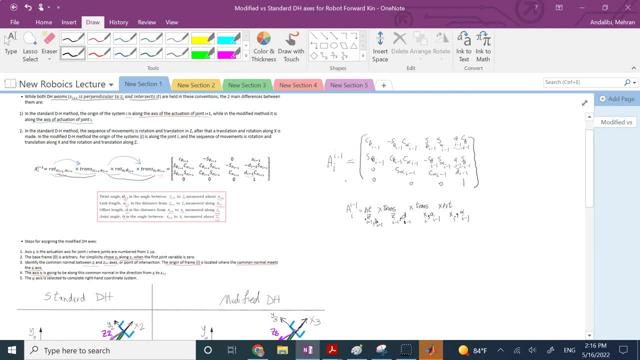 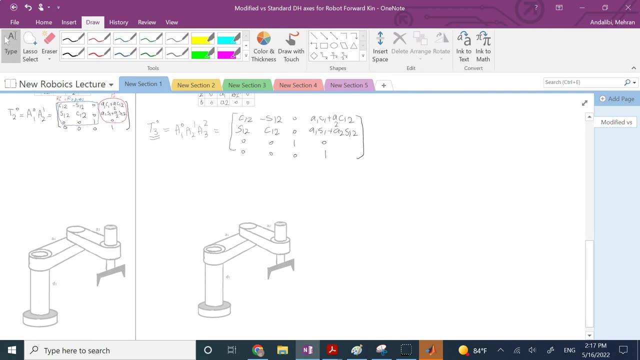 setup of axes and the number of them is different. the table looks different, the intermediate, a matrix, is different. the final result is not going to be in this case, because everything is the same. okay, so that's example. what number one that we talked about, the uh 2dof planner arm. the next example that i want to talk about with you is 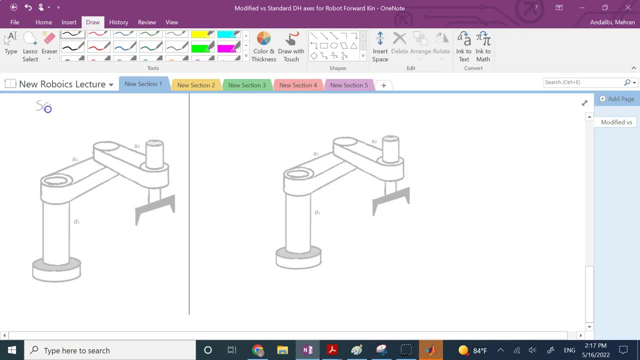 the scara robot, right that you know. and, uh, this time we only work with three degrees of freedom of that and we neglect the final spin. so the real rotations, uh, that you have are only theta one here and you have theta two here, and then you have this distance here that you might call d3 or q3. 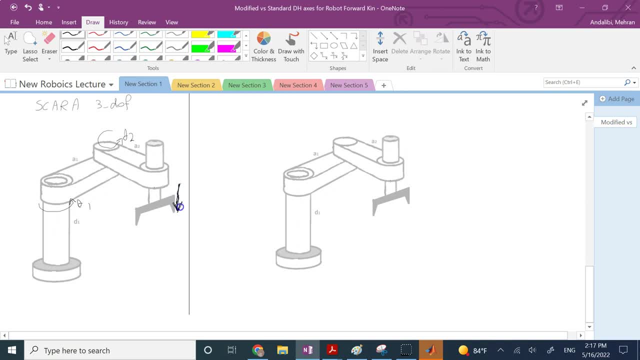 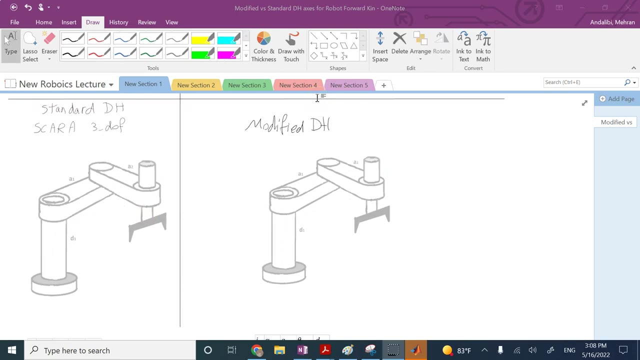 or whatever you might want to call it, which is downward positive. i call it d, number three, right, so we use only the three degrees of freedom of scara and we neglect the final spin of here that you can have. okay, let's go ahead and set up the dh axis. 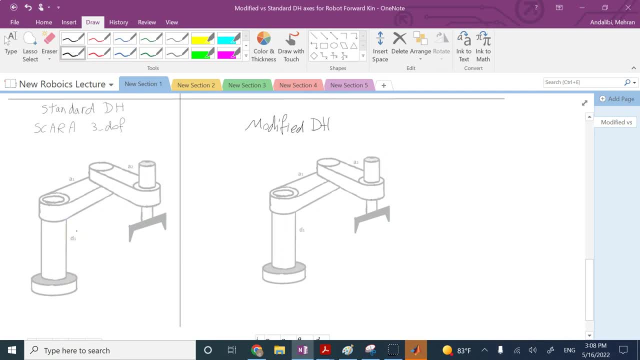 for uh, each link. so, uh, as you know, this is your joint number one, so your z zero should be aligned. this, basically axis. this is joint number two, so that's where you have to basically put your z number one. and uh, this is joint three, so that's where your z number two goes, right. 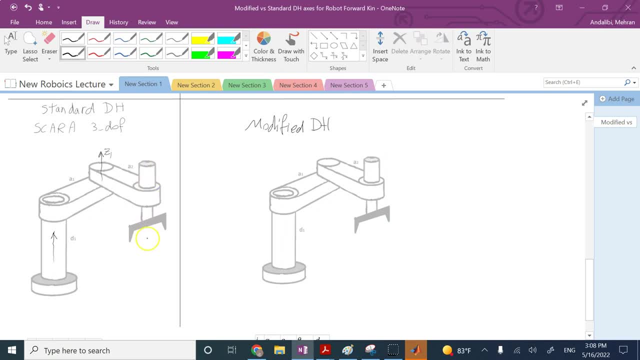 and finally, you have an end effector. and uh, here, uh, let me put z2 downward, as we just did for q three. and uh, you have an end effector. of course, the end effector. if you watched one of my videos when i talked about the ds axis, i guess it's the first one i talked about the ns. 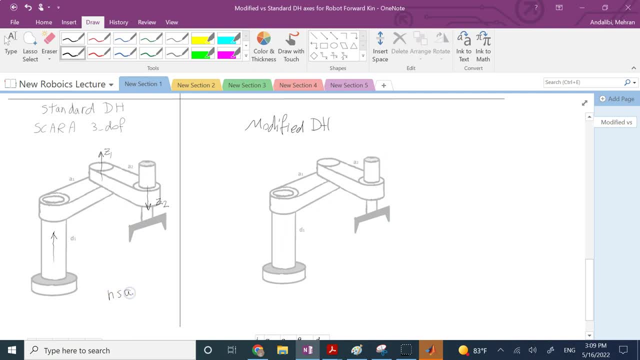 a or a and s. approach it's a combination of these three letters, so approach is the direction that the gripper- if it's a gripper- is going to reach the object, as s is the slide, the direction that the gripper is going to open and close, and n is normal to those and we typically go and assign z. 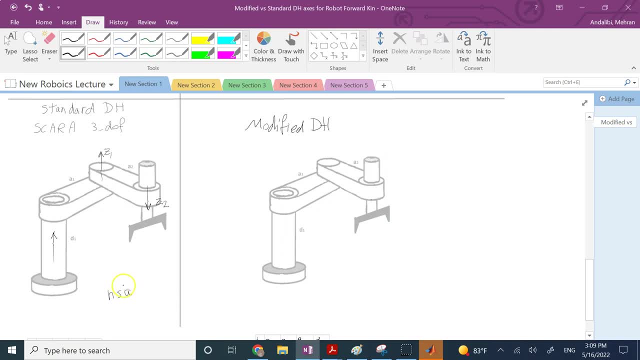 to a, y to um s and x to n. okay, but for here, since this is the direction of approach, so i'm going to put z3 here, and so my z's are assigned. and now it is time to talk about the x axis and the y axis. so first frame, 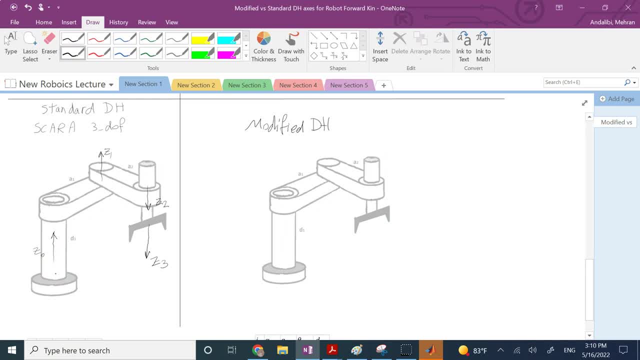 is frame zero. it's completely arbitrary. you can leave it wherever you want. the origin of it also do is um, since i know i would assign my x1 align the number one, so i'll choose my x0 to be similar to x1 when, except for the amount of rotation, it has right. so if this is like the center line and 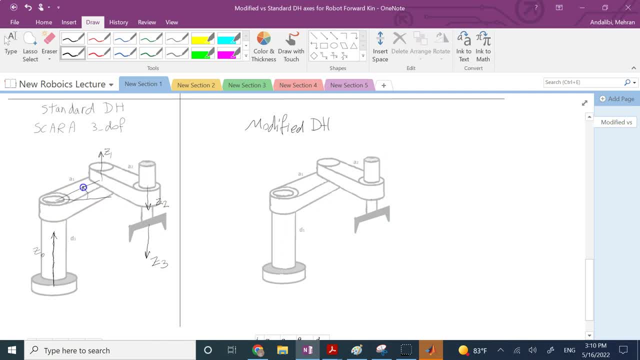 this is like the original x0, then this is like the angle theta one. so i make my x0 to be like this and this is to be y0. then i have to choose my x1 and i set it here at the origin. some people will choose the origin of. 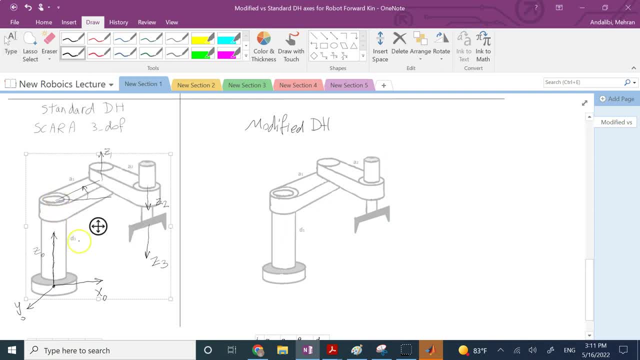 frame 0 to be here on the top and that way they can neglect this offset d1 in their final kinematics equations, you. But since i want to include d1, so i choose my origin down at the place where the base meets the supporting plane, like a table or something. then x1 has to be perpendicular to z0 and intersecting. 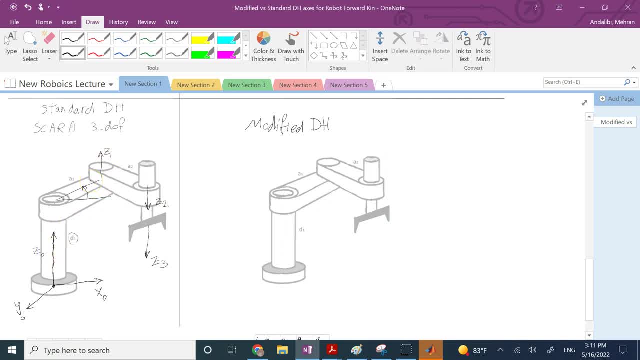 at z0 and z1 are parallel, so any line normal to both would work, and we definitely, since we want the two axioms to be correct. so we'll choose this direction and this direction is going to be my x1, which clearly intersects z0, and perpendicular to it, a line member number one and, of course, uh, we. 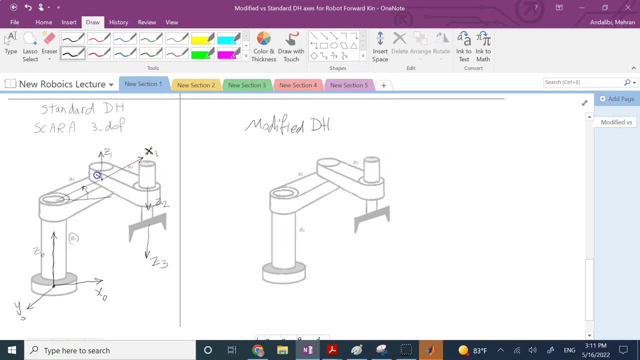 need y, so y should be in this direction. then i assume right. and again, as i said, this angle here is your theta number one, the angle between x0 and x1. then we come to x2. two again, z1 and z2 are parallel, so any common normal uh would work, but we wanted to intersect. 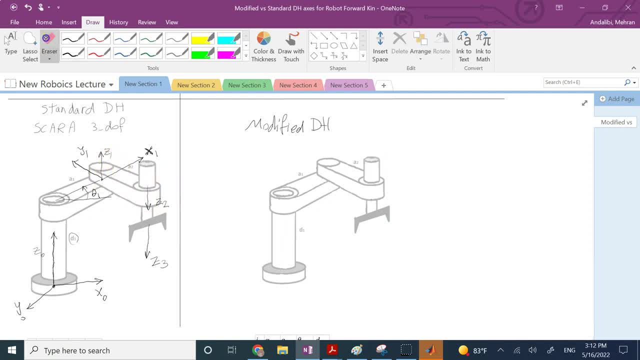 z1, so it has to be a line member number two. so for that reason, uh, i choose this direction, which is the direction of the member. let me shorten it a little bit to stay on this side. this is gonna be my x number two and, as we had downward direction, that was my uh z number two. 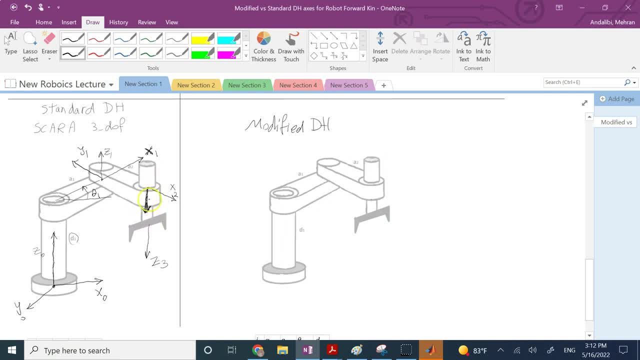 right. or if we want the downward direction to be uh, negative, then we have to choose my uh z-axis to be upward. okay, so it. the only thing it does. this upward or downward direction of z2 makes your third parameter positive or negative. and uh, here, uh, your x has to be your y- sorry, has to be in this direction. 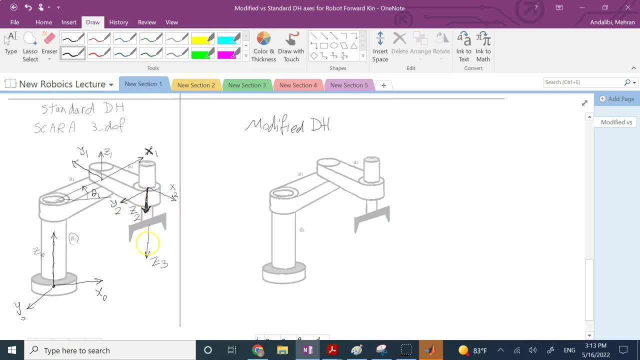 and now, uh, since this joint is only going up and down is prismatic, i'll try to align my x with x, so x3 and clearly three is in this direction, which is of course the direction of opening and closing the breaker, the slide direction. so you see, the slide is y, the approach direction is z and the normal to them. 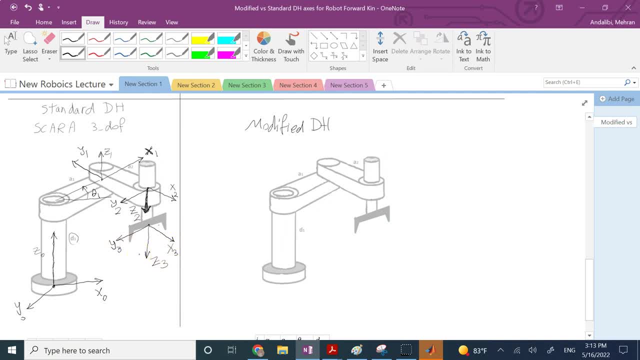 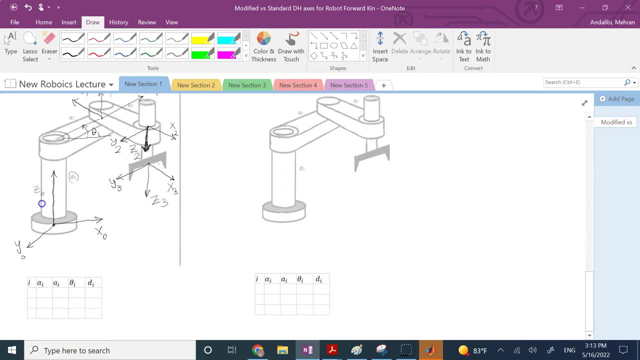 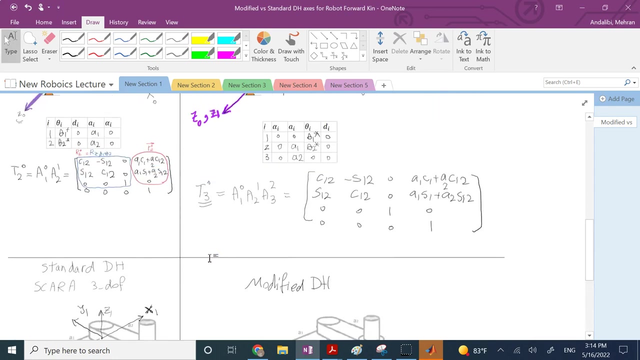 is x, so nsa approach definitely works for the end effector here. so that is my dh system here and if we want to fill it again, we have three rows because we have four axes and, uh, the order here. we just need to make sure the order is the order of the. 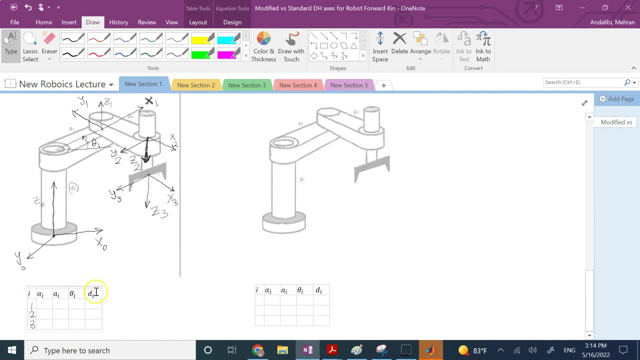 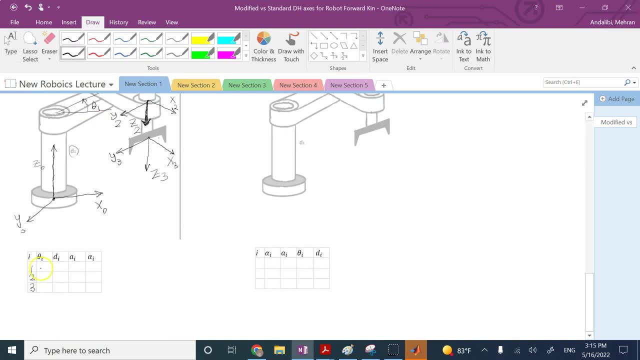 standard. so it's theta d a alpha, not the other way around. so here i fix it. and now, uh, as you know, the first angle is theta number one, which is your um joint variable. d is the distance you have to travel along along the old z-axis, which is the distance you have to travel along the old z-axis. 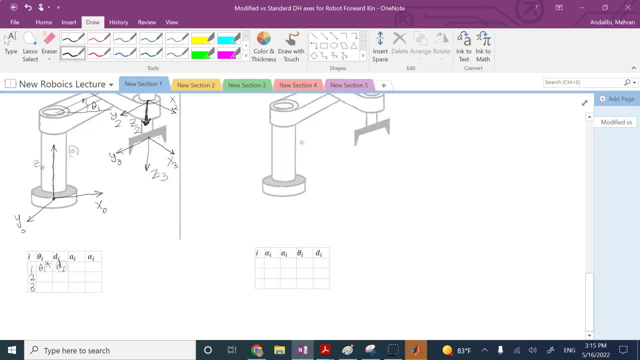 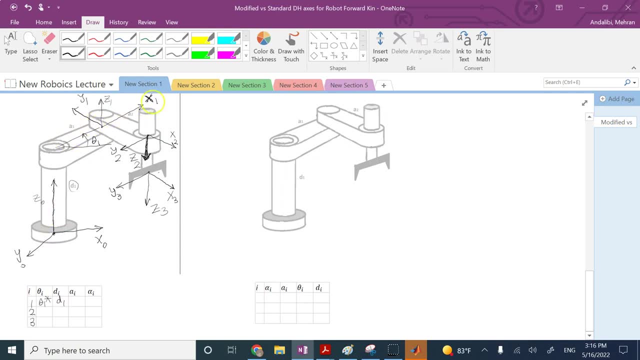 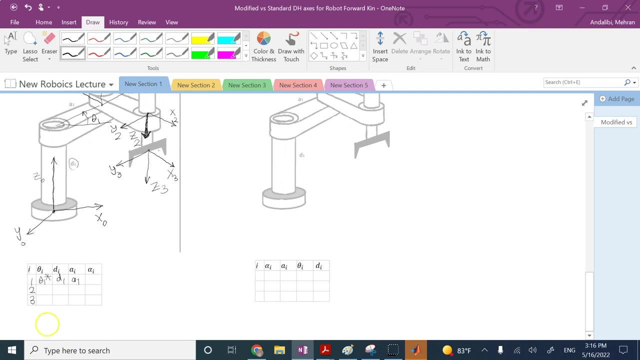 which is d1, and it's a constant parameter. and then you, when you go from origin of zero to origin of one, do you also need to travel along x1? yes, that's the distance. a1 and these of 0 and 1 are aligned already, so there is no twist needed. 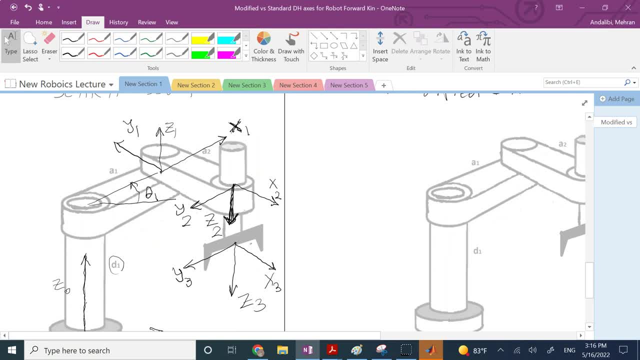 and then you go to the second one, then the angle between x1 and x2. you clearly see that if you draw this x2, this angle, theta 2 is negative or clockwise right, but that's what it is in this configuration. so theta 2 is your. 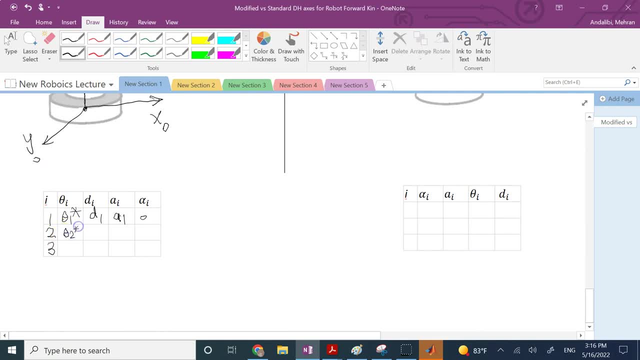 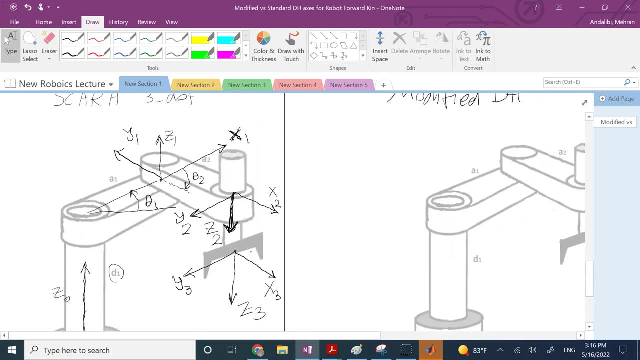 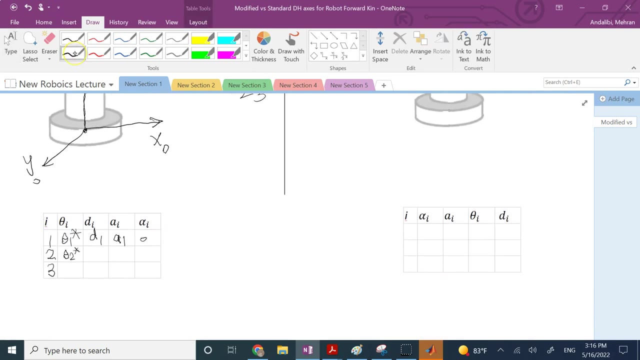 rotation, and that is again the joint variable. there is no D needed because origins of 1 and 2 are basically on the same level, on the same Z level, so no D is needed. your a is a 2 and your alpha in this case is 180 degrees, because your 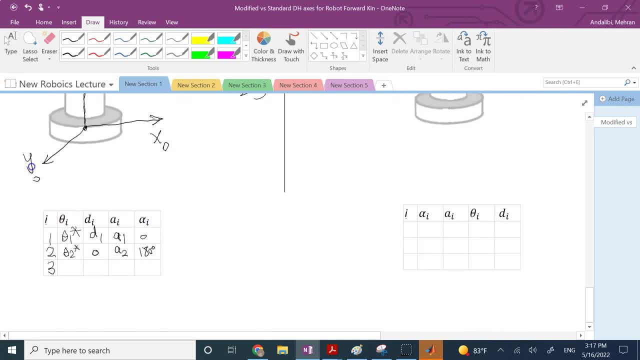 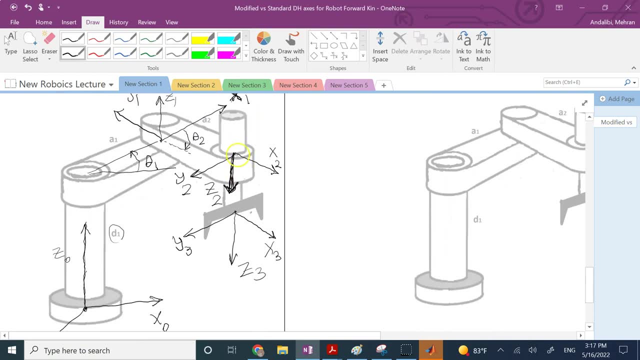 Z 1 is off and Z 2 is down going from 2 to 3. the X's are already down, going from 2 to 3. the X's are already down going from 2 to 3. the X's are already aligned. there is a distance aligned- the z-axis- that you need to move, and that is. 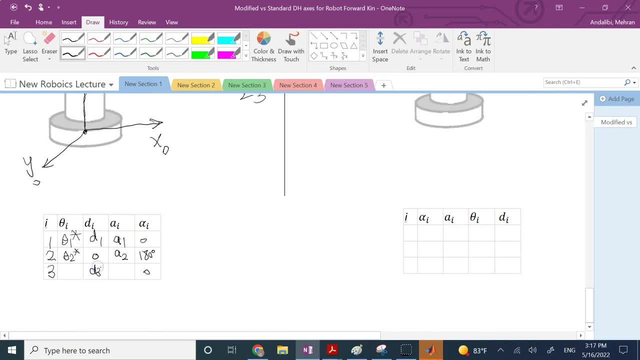 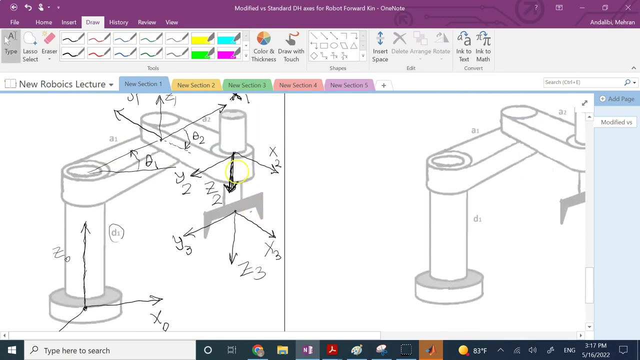 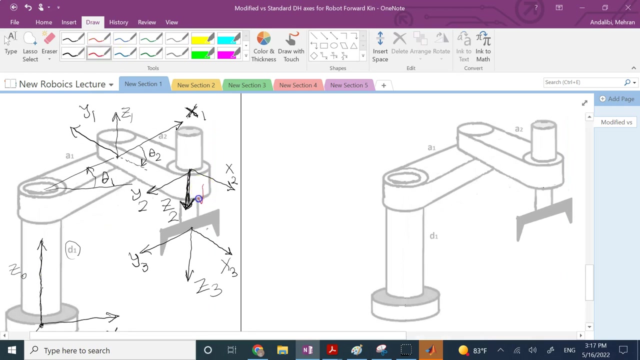 called the number three, or q3 you might call, and that is your joint variable. there is no detail need that the X's are also aligned and no, a no motion align. the new X is needed and d3 is clearly this distance aligned which this prismatic joint is going up and down. okay, so this is your D, H and 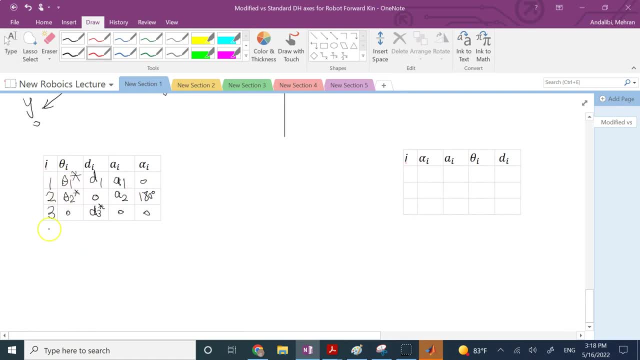 I'm sure you can multiply the A's coming from them and get your T or T of three with respect to zero, which I have covered in one of my previous lectures. so I'm not going to do that, save the time- and I will cover the modified axis. 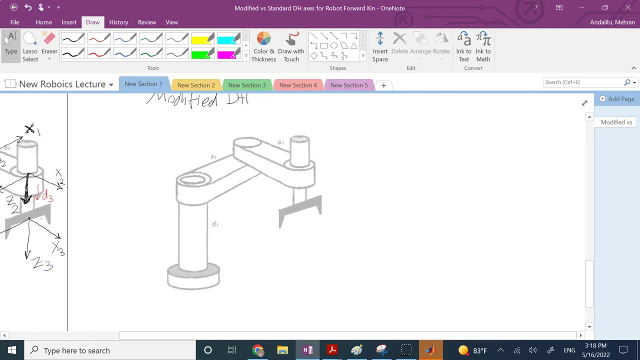 for these, this 3dof robots. so in this case, if we want to talk about it, you need to make sure that your Z's are matching the joint. so this is joint one. therefore, definitely it has to be Z one. this is joint two, so it has to be Z. 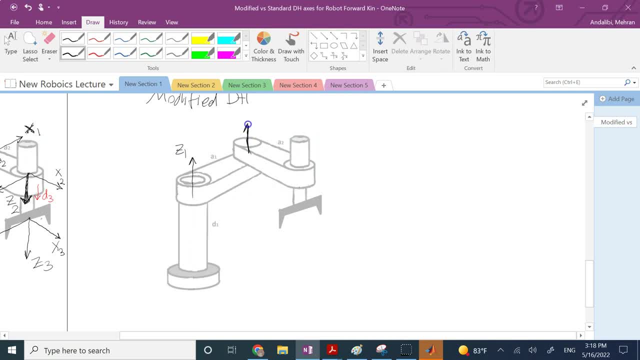 number two, and this is joint three, so it has to be Z three again. you can make it up or down. in this case I'll choose to go down, like the previous case. right, and you can also. if you want, you can also bring your Z three and put it here at the end effector. 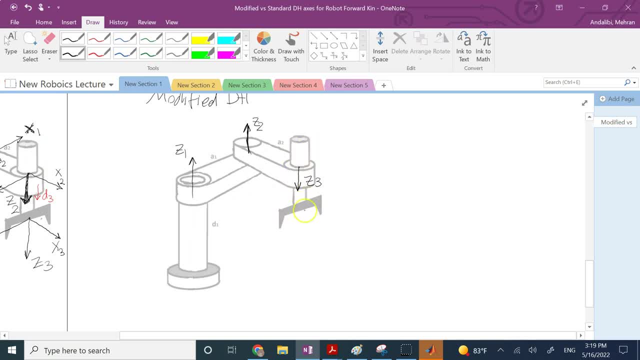 because- and this end effector is attached to this member that is going up and down. so there is really no need for me to add a fourth axis and call it Z four. if I want, I can really bring this Z three and put it down here right to show that I need to go down that distance of D three. so 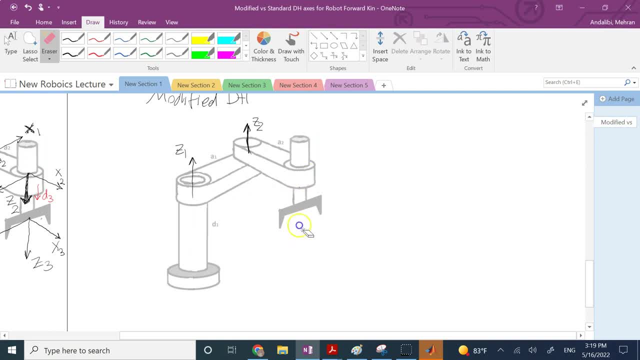 I'll, or that's basically the location of the origin of it that matters and we're going to cover next, but I'll put it down here. okay, and now we're. what about Z zero? again, it's completely up to you. you can choose, as I said, Z zero. 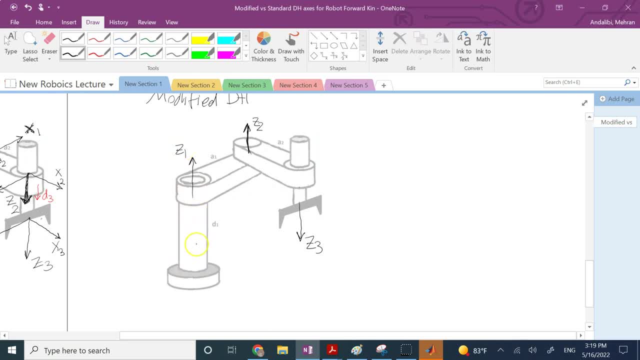 to be the same as Z one. so I'll choose this upward direction to be Z zero. but I'm not going to put the origin of frame zero at origin of one, because I want origin of one to. as you'll see, I want it here, so instead I'll put the origin of zero down here and again. the only reason. 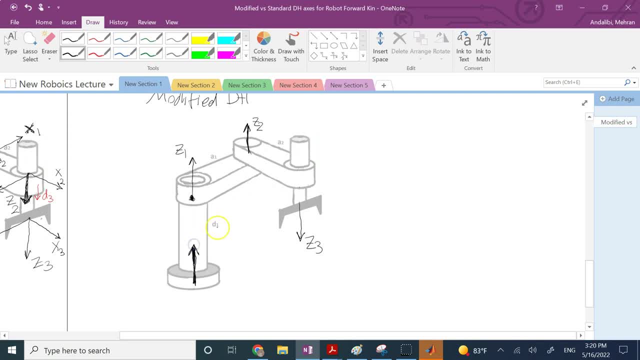 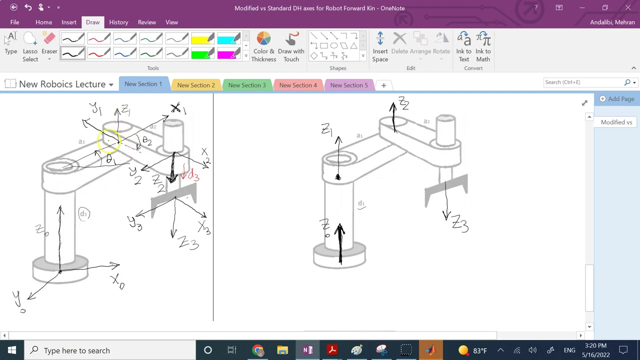 for it. I want to include this parameter D1 in my forward kinematics. so I choose my Z zero on the origin of it, on a separate location, but still you see Z zero and Z one are on the top of each other and still I gonna go with um X zero such that is perpendicular to Z one and intersect in it. 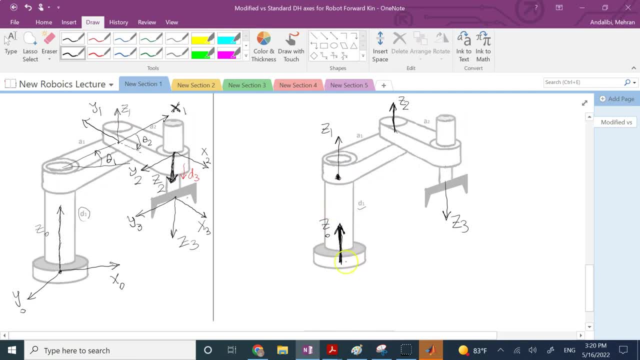 and Z zero and Z one are on the top of each other, so any vector I choose would work. really, I choose the same um X that I did for the standard, and this is Y- zero. now when I go to frame one, the new X should be aligned the common perpendicular to Z1 and Z2, since they are parallel and you need your X1 to. be cutting and perpendicular to Z two. so that's what I decided to do, and you will see that at the end of this video I'll also do some- just some- interesting work on this thing that we should be doing, and then we'll be doing some pretty basic stuff now in the block. 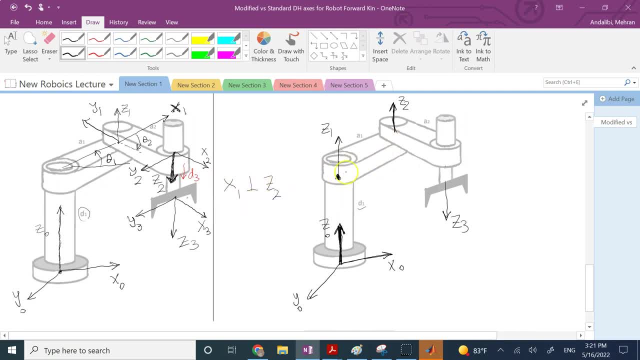 z, number two, right, so you choose it. align the member. so you choose it this way and automatically that means your y one should be in this direction and now your x2 that you choose, should be intersecting and perpendicular to z3. again, z2 and z3 are parallel to each other, so i still choose it to be align this member, so that is. 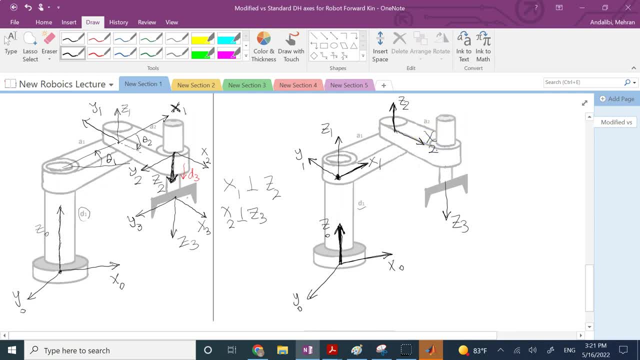 going to be my x number two, and that x and that z would imply a y outward, like this, and then it's down to z3. so now, uh, i need x3. x3 is going to be perpendicular to z4, but there is no z4. 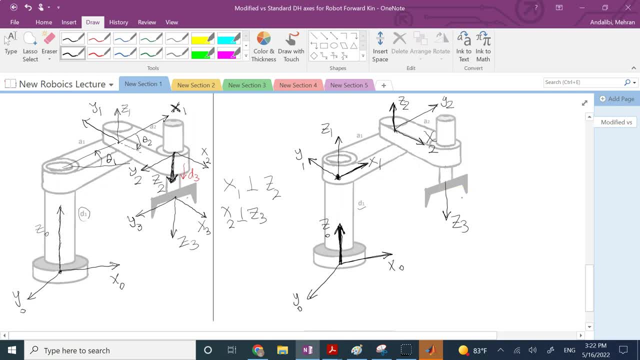 so really, here i can choose the direction of x3 and to minimize the amount of non-zero parameters. i choose x3 to match x2 in that direction, and this direction means y3 is going to be inward, like this. okay, so now you clearly can see the difference between uh, the modified and what the um. 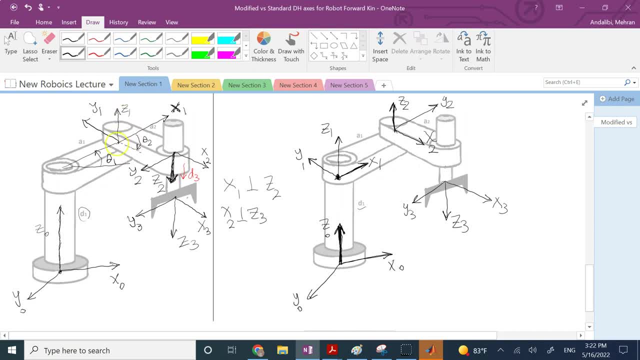 standard. as you can see here, joints one and origin one, z one and origin one are on joint two. z-one origin one: here they are on joint one right. or z2, origin two are on joint two. here they are literally on joint three right. so this kind of shows a better distribution of the. 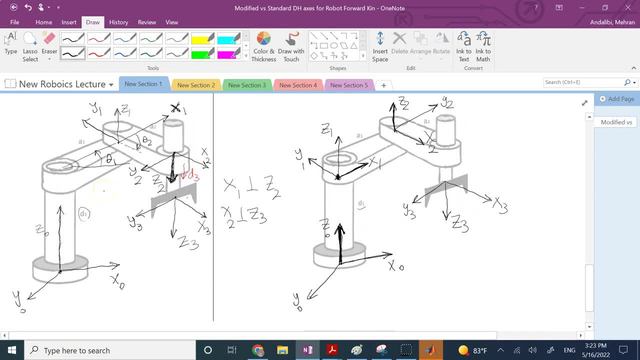 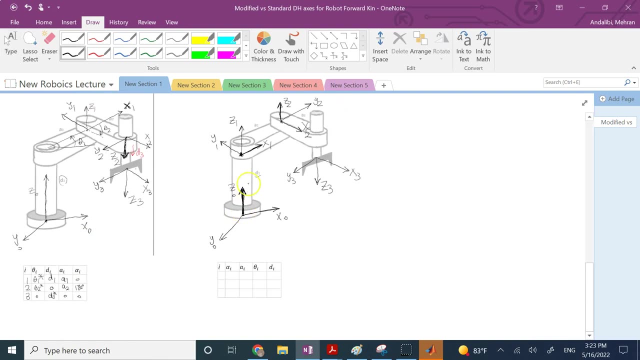 location of the axes instead of this one. but again, um, it's not like something very, very fundamental, but just want you to know how they are going to be set up. so here if we go, when you go from frame 0 to 1 and remember the order, 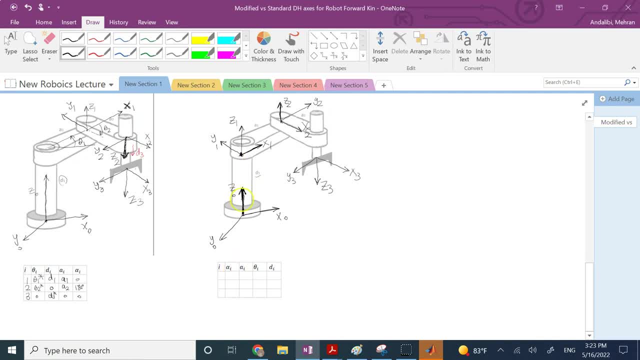 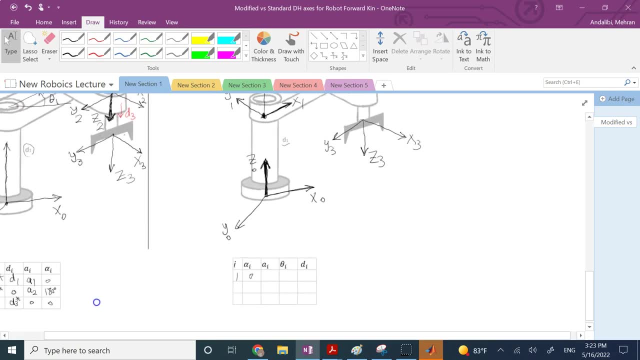 first you have to twist about the x-axis to align disease. but disease are already aligned, so no twist is needed. and then you have to move along the old X. you're not going to move, they are allowing the same Z direction. then you have to rotate about the new Z, which is Z 1, to align X naught with X 1, and that angle as we 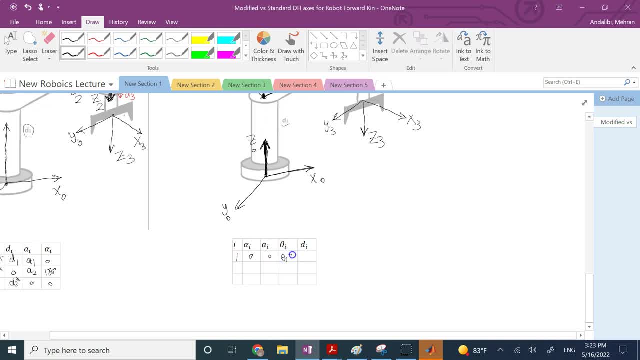 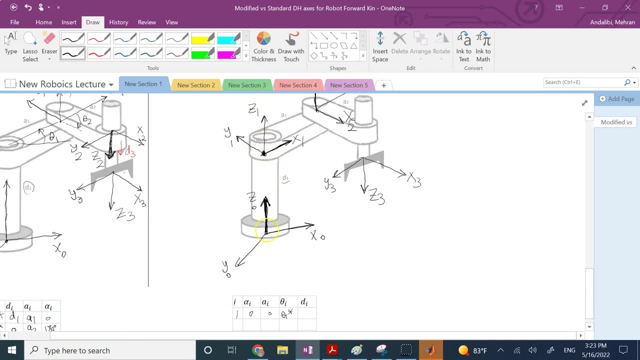 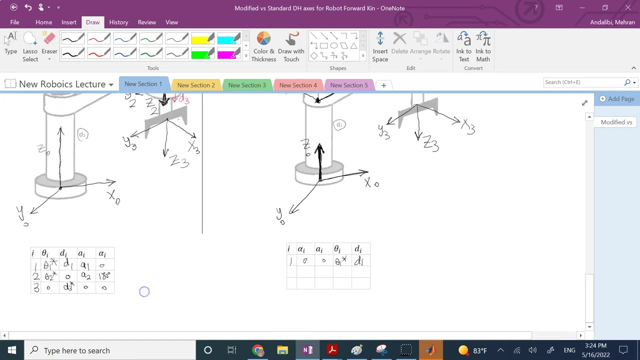 discussed is theta number one, which is the joint variable, and do you need to move a line get this Z 1 direction to go from origin 0 to origin 1? yes, that's, distance is called D 1, so this is the first row, which is the exact same thing. 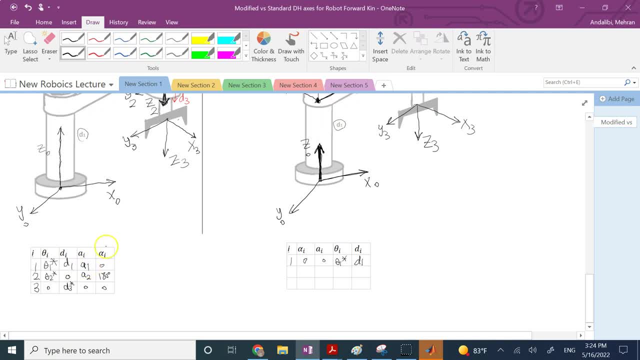 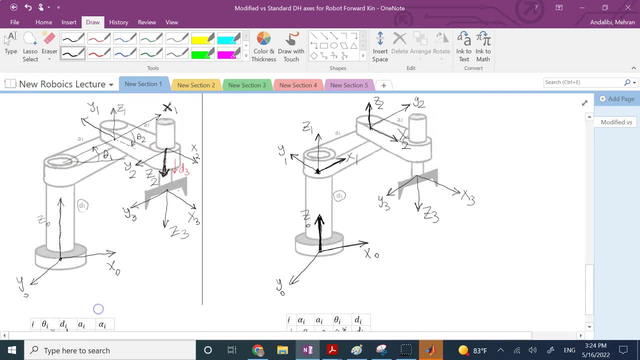 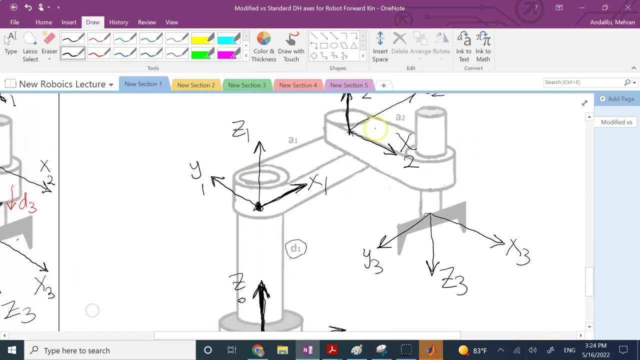 as that one, except for a 1. the way that origin 0 and 1 are set up, there is a 1 here. that a 1 is not included here, it will be included in the next row. so now I go to 2 and 2. here is between 1 and 2. clearly, disease are already aligned. 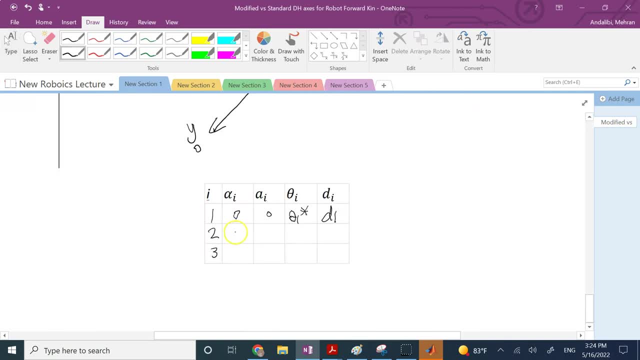 therefore, I don't need any rotation. do I need to move a line? the old X, X, 1? yes, that distance is called a 1. do I need to rotate about the new Z? yes, that angle is called theta 2, which is the joint variable. they are both at the same. 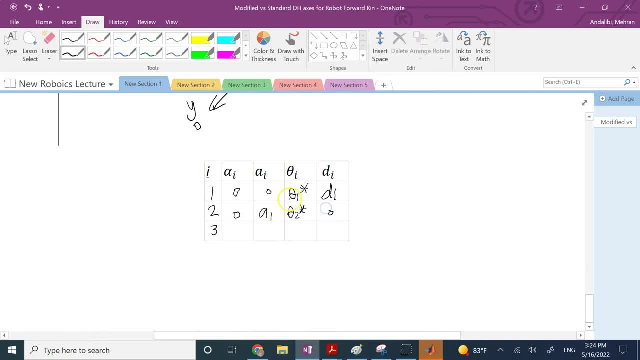 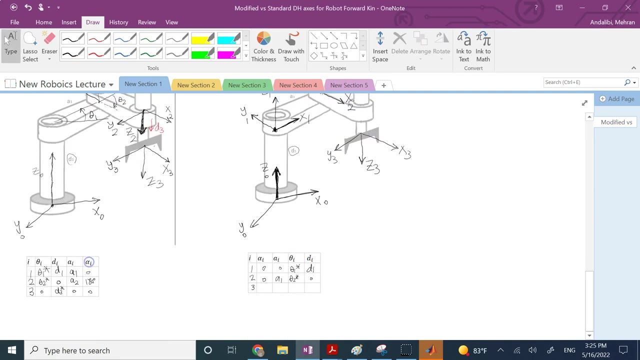 Z level. therefore there is no D needed. so you see now a 1 came to the second row instead of the first row, right, as you can see side by side. then, when you go from 2 to 3, this is where you have both a and D, right? you clearly first of. 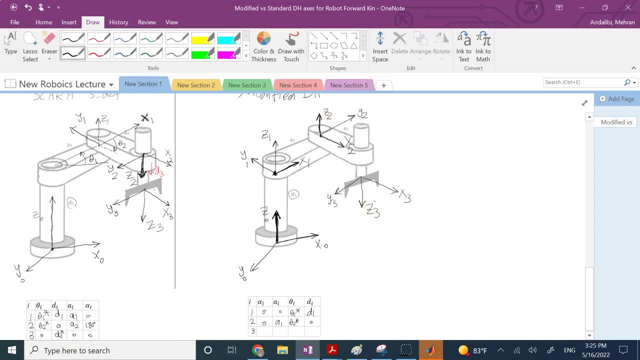 all. do you need a twist? yes, because Z 2 and Z 3 are in different directions. how much do you need to go from Z 2 to Z 3, that's if a rotation about X 2 is happening? clearly, that's 180 degrees. now it might be positive or negative. 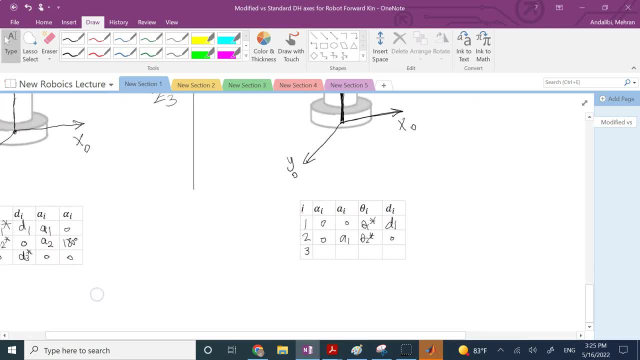 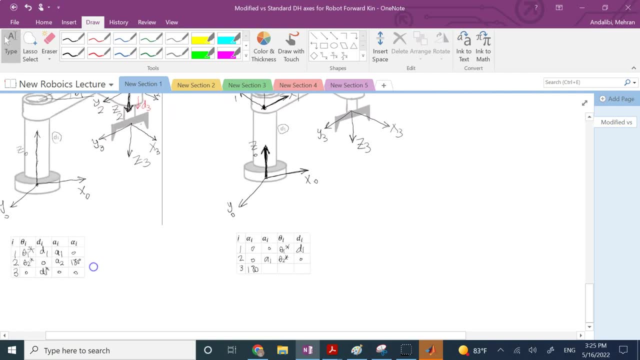 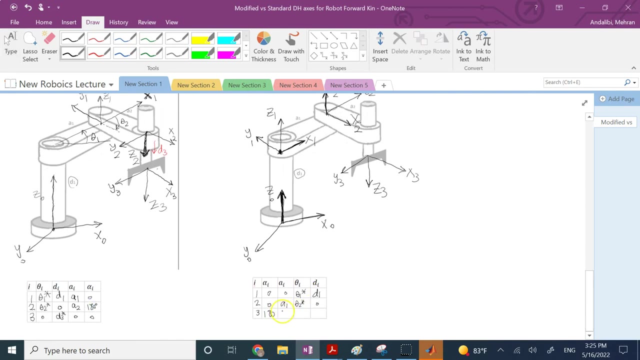 it's not going to change anything, right in the case of 180. whether it's positive or negative, the final result is the same. so the sign here, exceptionally in this case, doesn't matter. and a- yes, you need to move a line, the old X, so that is a 2 and there is no theta. 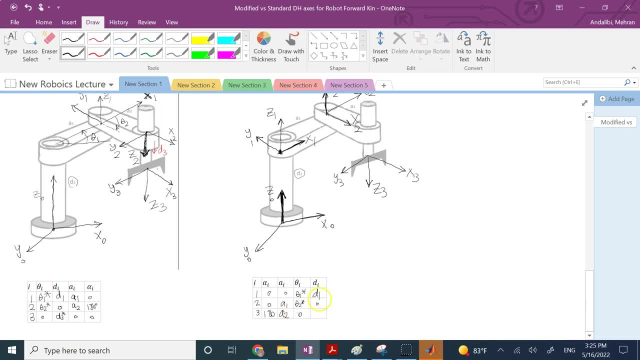 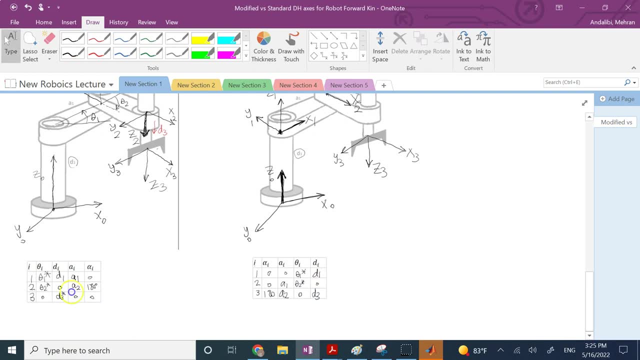 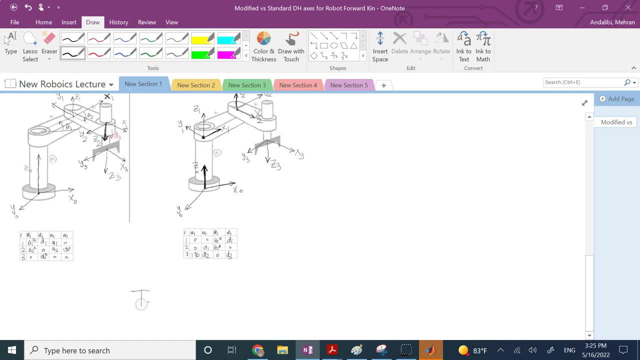 needed, because I chose X 3 and X 2 to be aligned. do you need to move down? yes, and that is called D 3 and if I go ahead and in this case, in both cases, calculate T of 3 with respect to 0, which is a of 1 in 0 times a of 2 in 1, times a of 3 in 2, the question I have for 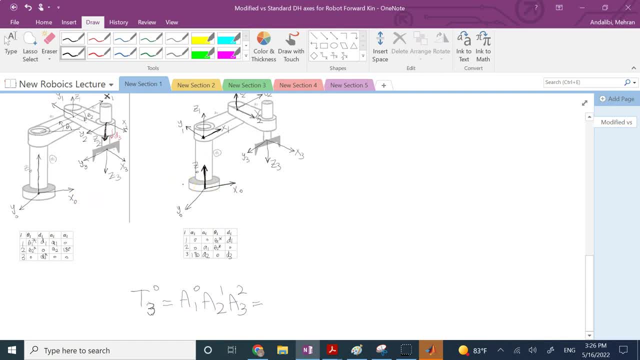 you? is that gonna be different for the left and the right side? given that the rows are different, the X's are different. would I get the different 4 by 4 matrix? the answer is no. why? because in both cases, as you can see, my frame 0 and my 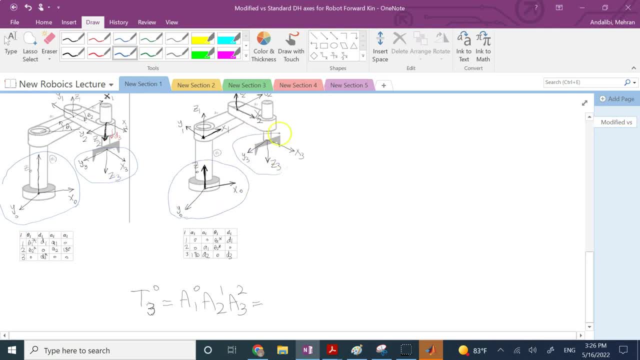 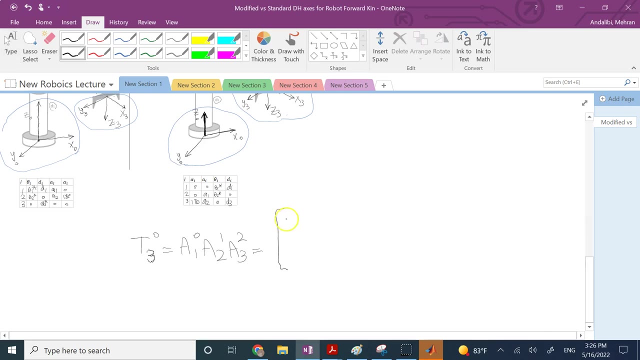 frame and they are the exact same thing, so I should not be getting any different presentation and indeed, if you do that, you are not going to get any difference. if you do that, this is going to be still c12 negative, s1, 2s, one, two, C 1, 2, 0 0, 1 0, 0, 0 0 0, 1 and the 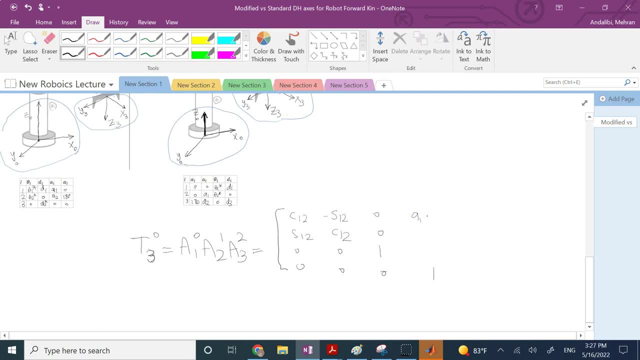 And then this is going to be A1, C1 plus A2, C1, 2, A1, S1 plus A2, S1, 2.. And then it is going to be D1 minus D3, and then 1.. 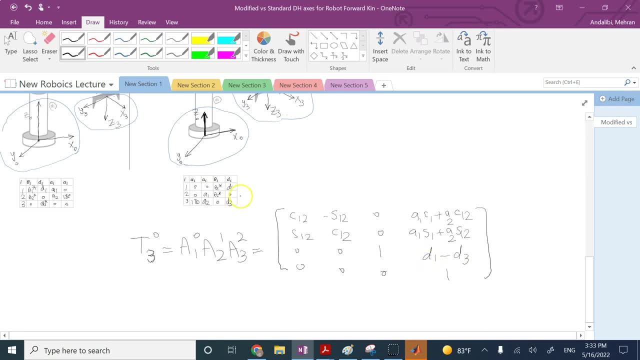 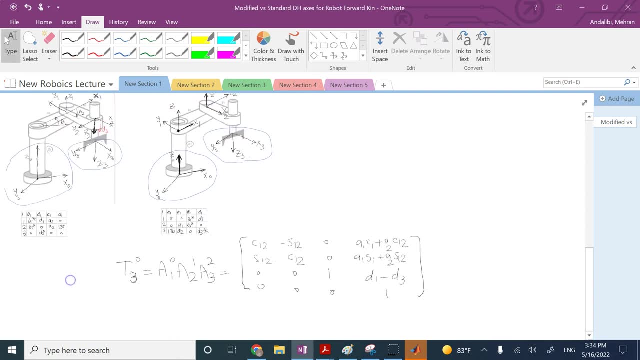 So the result is going to be the same, and this D3,, by the way, is the joint area. Okay, so this is for the 3DOF scara, It's for the 2DOF planar arm. 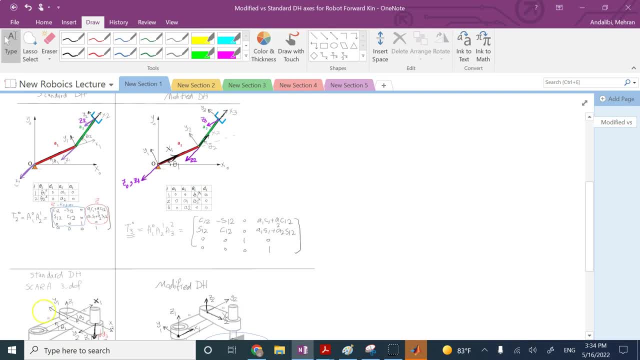 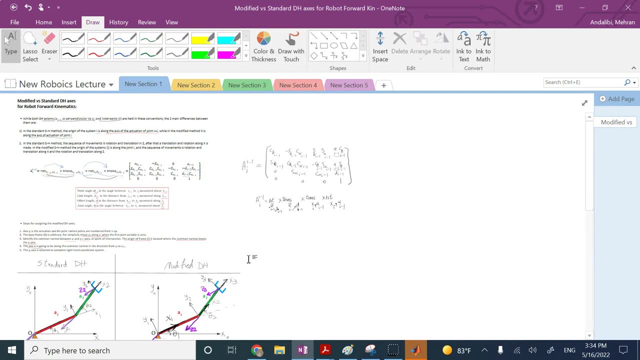 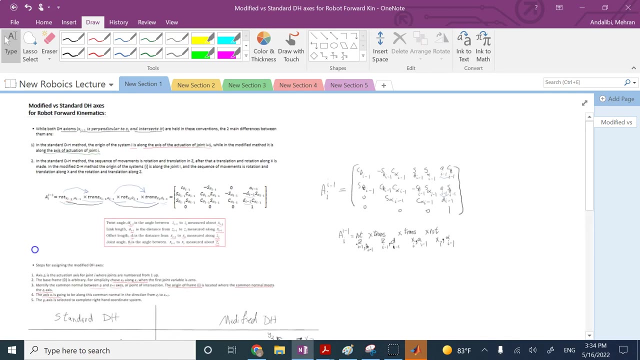 You see, the X's are different, The intermediate A matrices will be different. but depending on whether the first and the last frame are the same or not, you might get the final T matrix to be a little bit different or not. But clearly the modified method will overall- you might say will- make a little bit more sense. 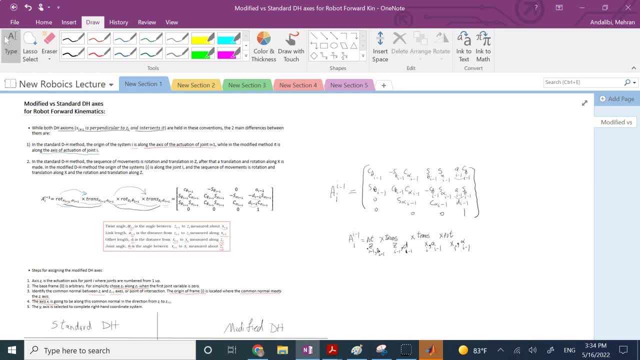 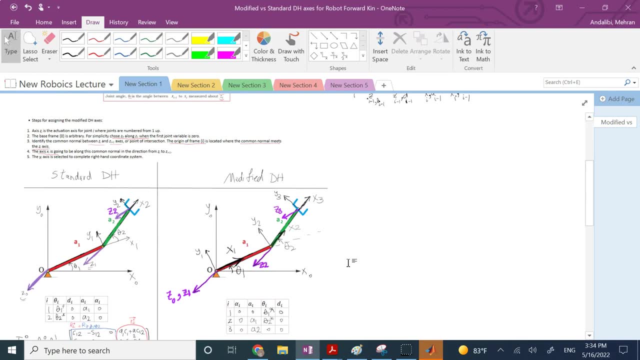 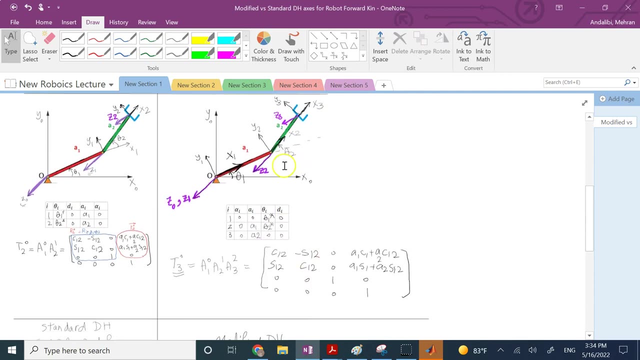 since it puts the origin of frame I on joint I, not on joint I minus 1, or I plus 1,, really Okay. but sometimes, in this case, like you see, you have to provide an additional frame to include all of the parameters and get the same result. 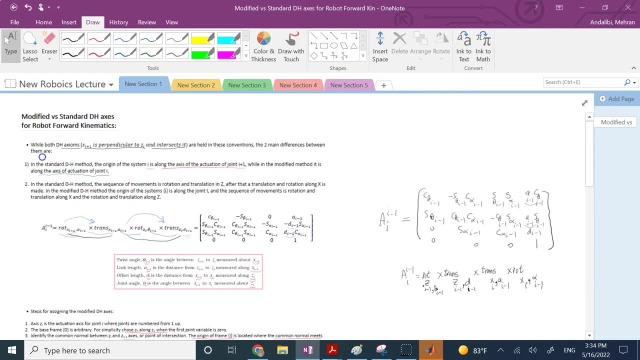 So hopefully this video was useful to you and I will see you in my next lecture. Thank you.